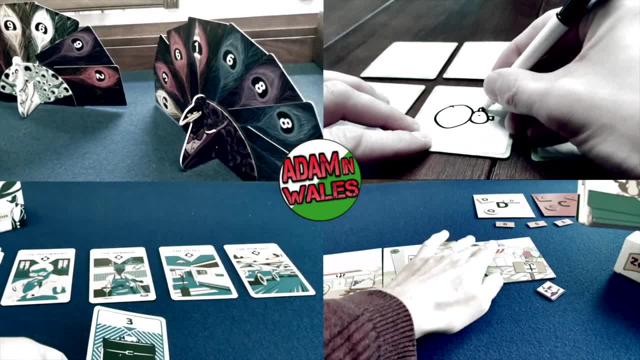 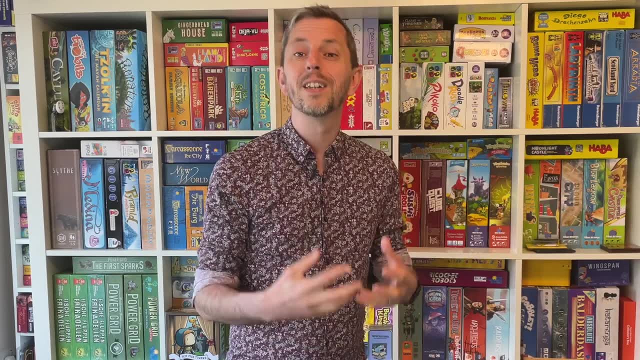 my experiences in the world of board game design. If you like what I do, please subscribe, comment and share the video. This video is really intended for those first-time designers who feel a little bit lost with the process of creating the game. I'm not saying you can't get your hands on this. 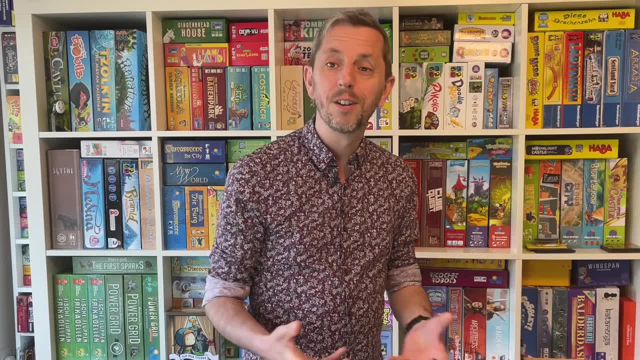 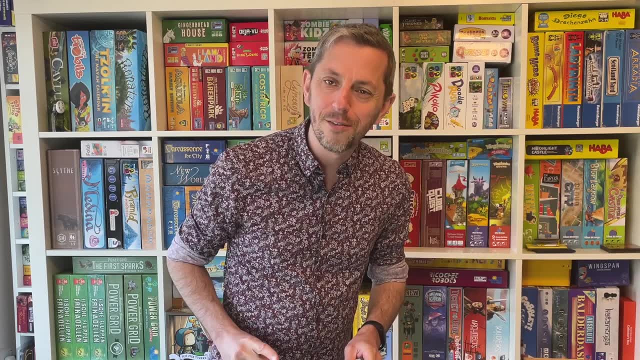 of board game creation. I receive emails from such people on a regular basis, and the question tends to take one of two forms: One: I want to design a board game, but I don't have any ideas. Or two: I have an incredible idea for a board game, but 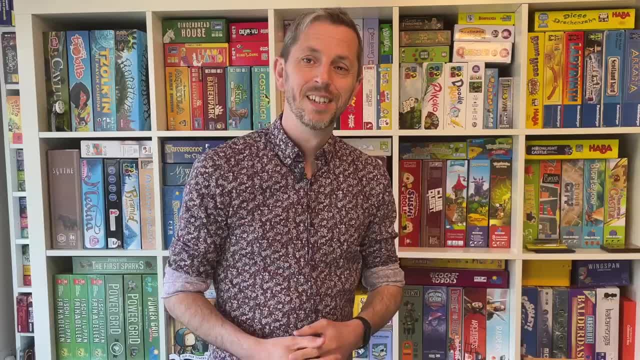 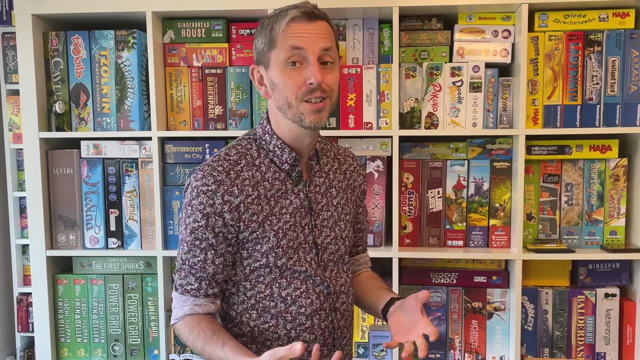 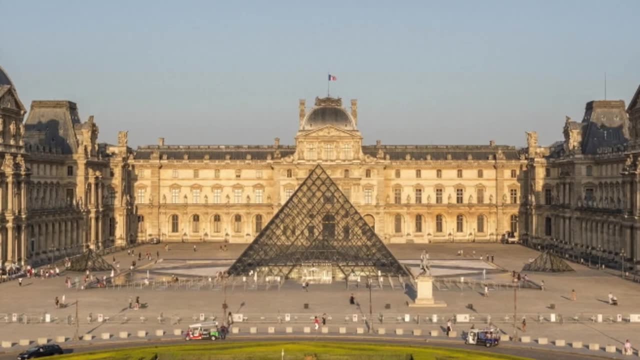 it's all in my head and I don't know what to do next. Now there's no right answer to either of these questions. Those first tentative steps as a game designer are perhaps the most personal, the most dependent on your own personality, tastes, experience and priorities. Fine artists don't hang their 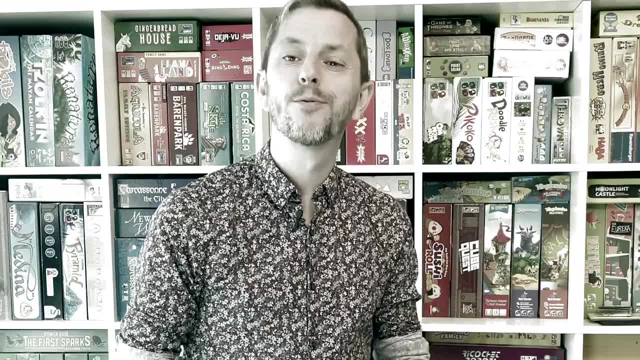 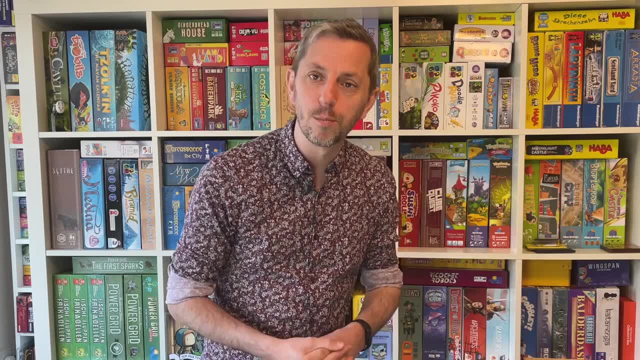 first ever painting in the Louvre. It goes on their mum's fridge. World-renowned novelists don't publish the first stories they ever penned. They're jotted in the back of an exercise book. awarded a gold star by teacher, Perhaps not even. 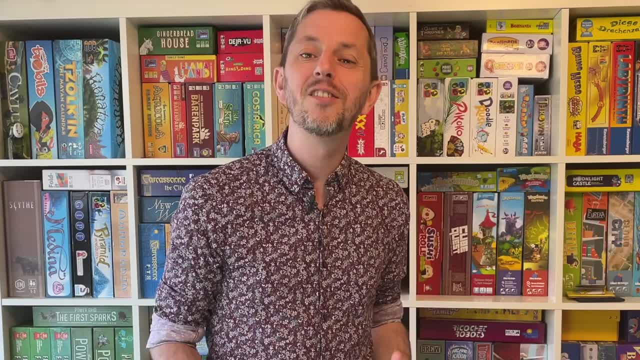 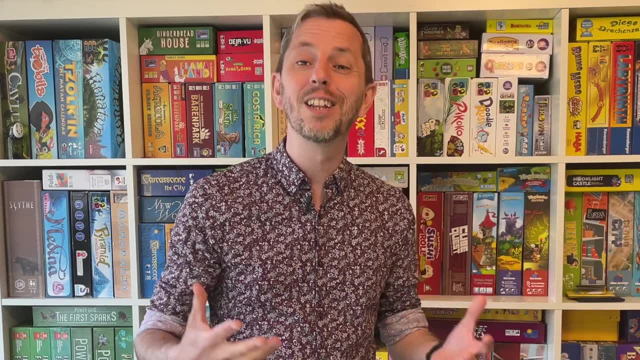 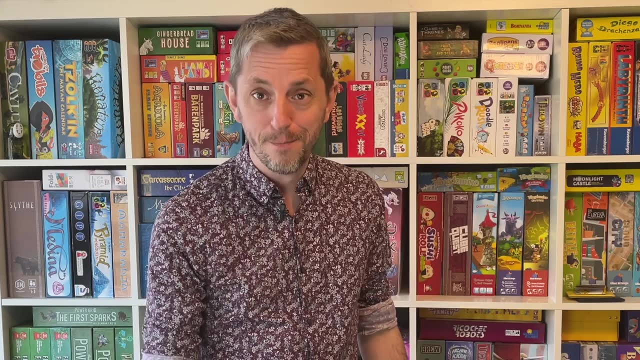 that Game creation is the same. Your expectations for your early designs should be low, But you should enter into these experiments with a wide-eyed, childlike interest. Game ideation is a joyful process, So start out by chasing the fun. I was a game designer all my life. I just didn't realize it. I remember. 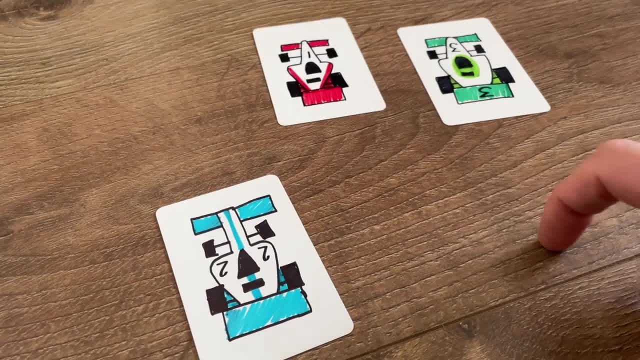 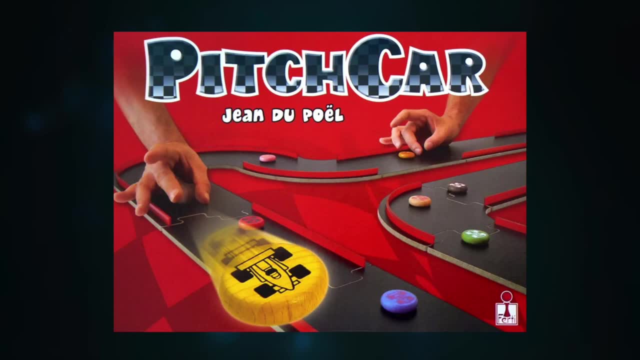 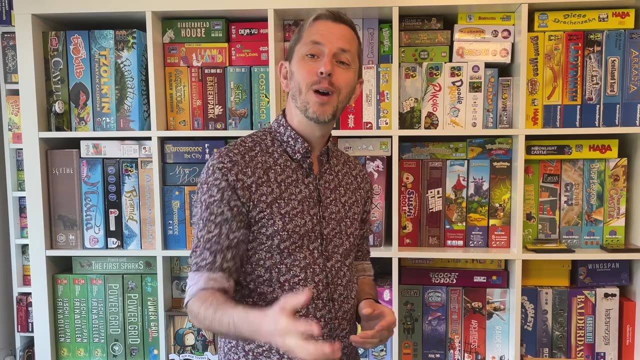 drawing racing cars on tiny pieces of card and flicking them across the living room floor, completing circuits around the furniture. I invented pitch car at eight years old, some ten years before Jean de Paul won the Spiel des Jahres with the same concept. At the age of 12, I got hooked on the idea of a board game. 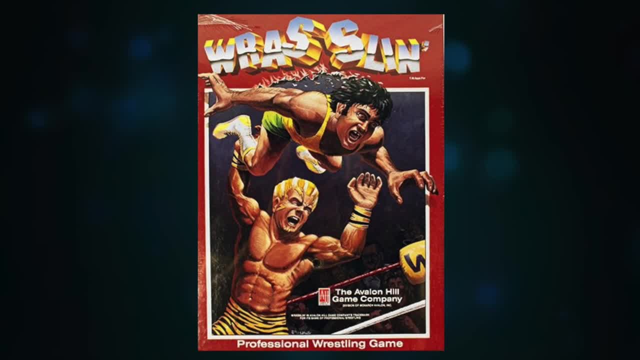 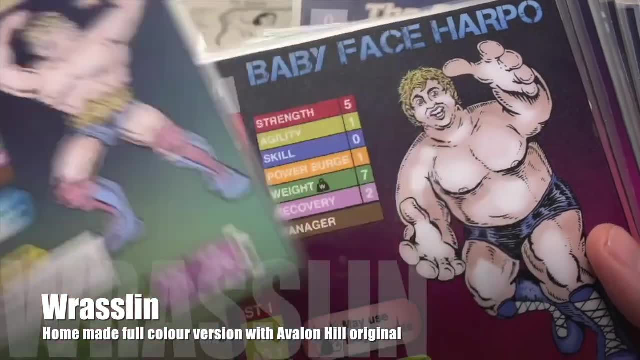 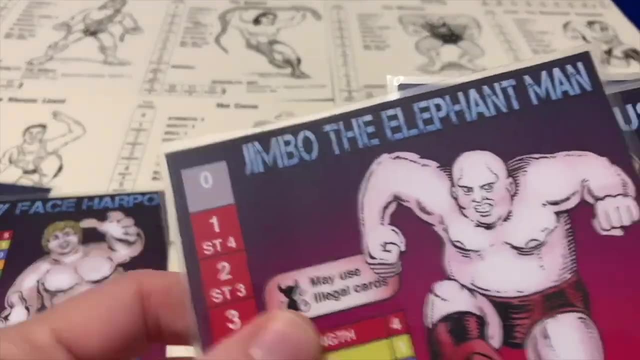 A simple take, that card game simulating the Hulk Hogan era of American wrestling. But I wasn't content playing the game in the box, Mimicking the play-by-mail football leagues my older brother was obsessing over at the time. I created a wrestling league. 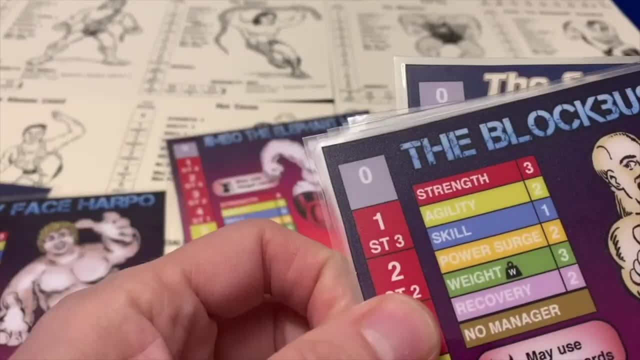 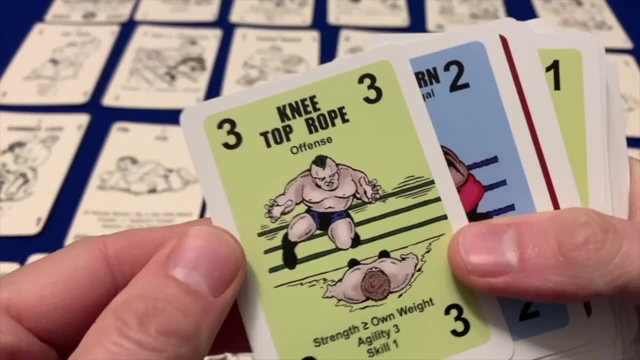 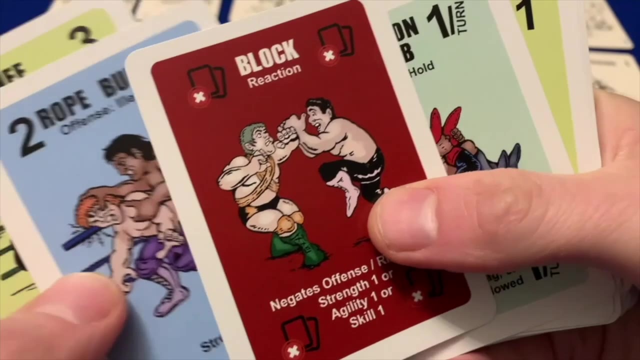 for my friends. I made a character generation system inspired by the one I'd read about in Palladium's pen and paper. RPG Heroes Unlimited. Our wrestlers upgraded their stats and signature moves. They suffered injuries, formed friendships and rivalries, switched allegiance and evolved from one match to the next. I loved creating worlds for. 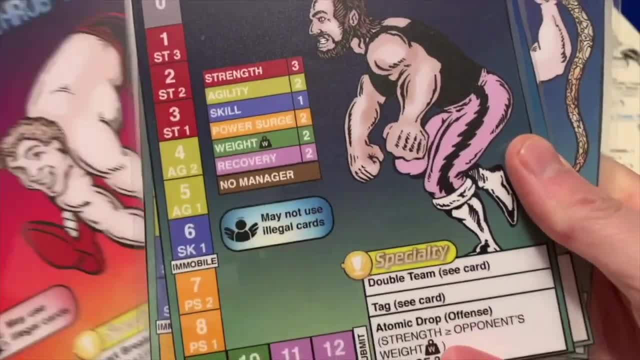 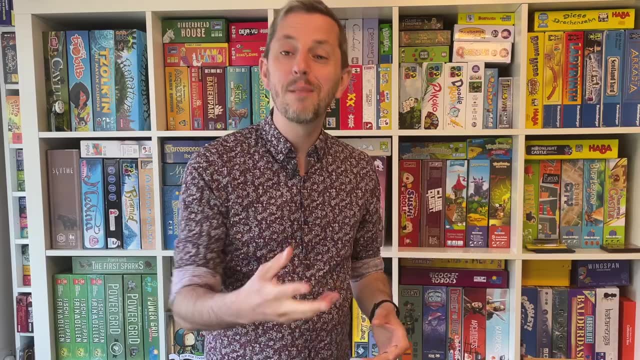 my friends to play in. The rules weren't balanced. Most of the time there weren't any rules. it was all off the top of my head. I was chasing the fun. Like any creative pursuit, game design shouldn't be a chore. It should never be forced. 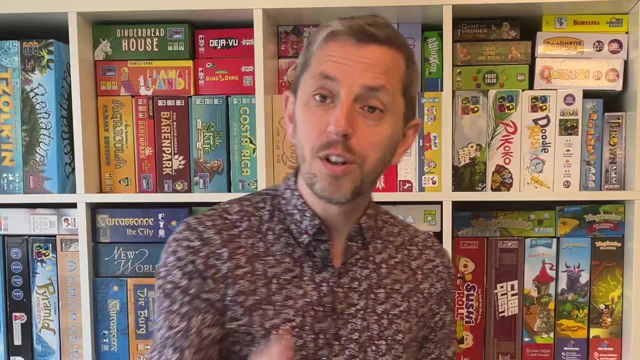 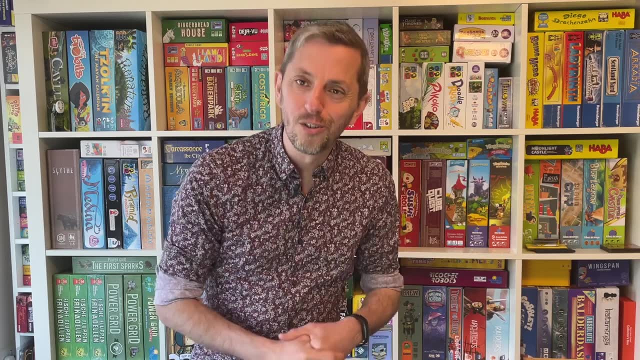 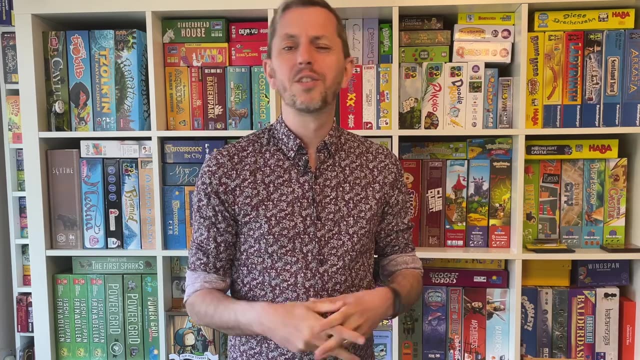 The process should be organic and easy. So what do you need to become a game designer? An attitude, active, playful spirit and someone who will indulge you, a willing guinea pig to try out your half baked ideas. When I was in my early 20s, my sister was seven or eight years old and I loved hanging. 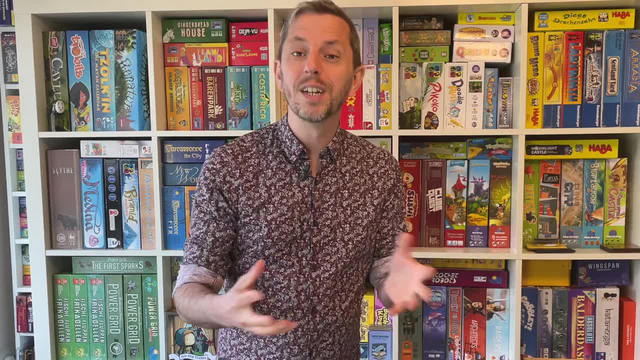 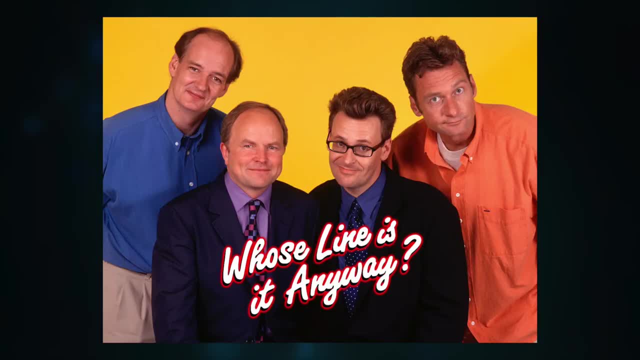 out with her and encouraging her to be creative. I was running an improv theatre group at the time. My mind was often occupied with creating new drama games. in the mould of whose line is it anyway? My little sister had an enormous, expanding collection of Thai beanie babies, animals of 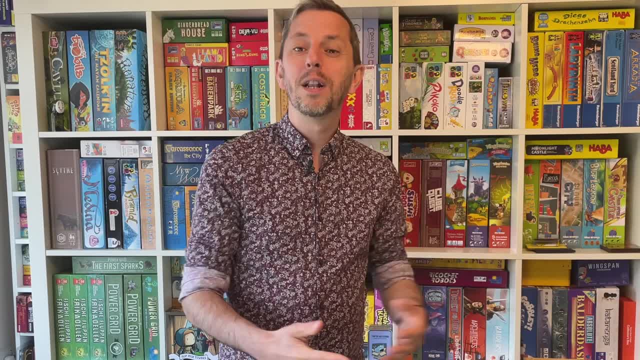 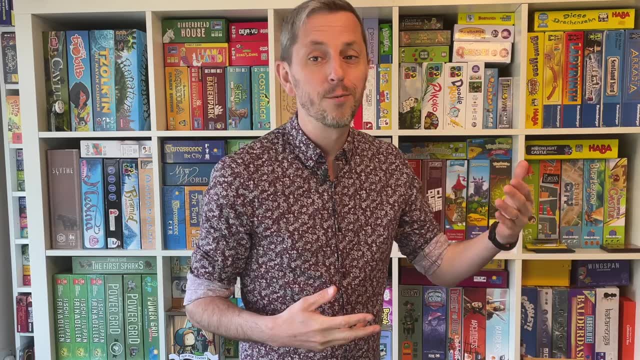 all varieties and colours, and together we developed a rule set for racing beanies across the living room floor, just like my cardboard racing cars, except these racers weren't flicked. Their moves were dependent on dice rolls and measured out with a tape. They could attack and defend too. 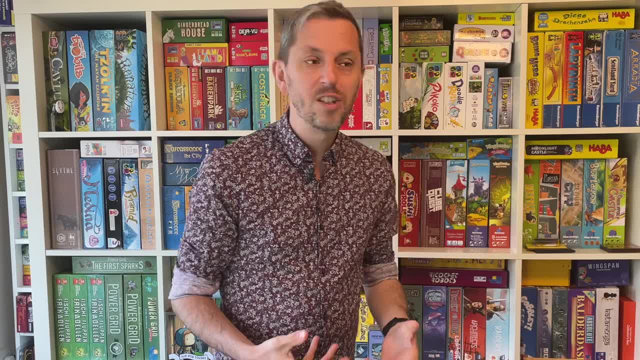 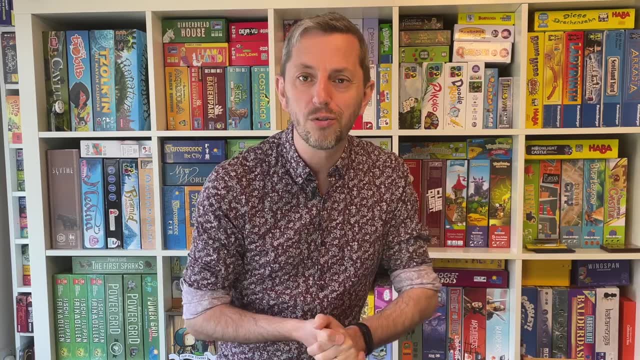 and each racer had its own traits depending on its species. So horses had a boost for speed, dogs had an attack, and so did the racers. There was an attack bonus when fighting cats. Winged animals ignored difficult terrain and each animal would. 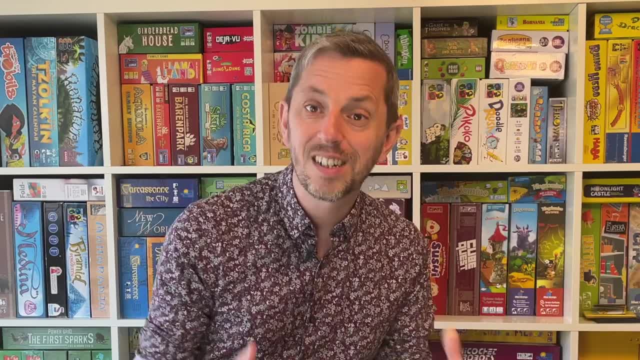 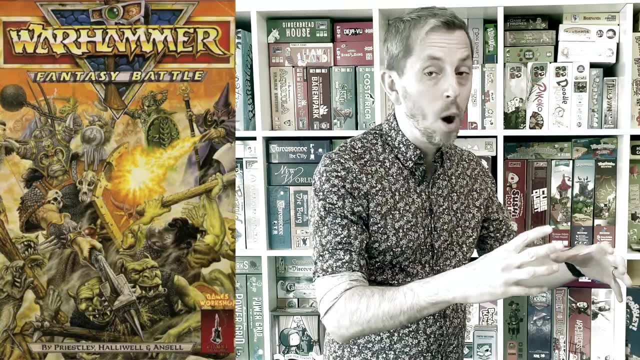 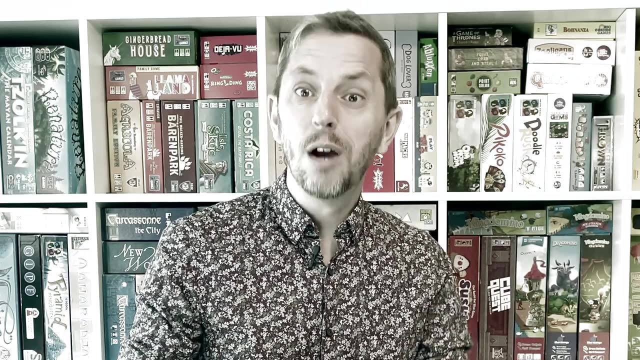 level up depending on the outcome of a race. Their stats would change and they'd develop new skills, all recorded in a little notebook. This was Warhammer meets D&D meets plushies, and we played for hours. I still didn't know that I was a game designer. These are the scrawls of a nascent. 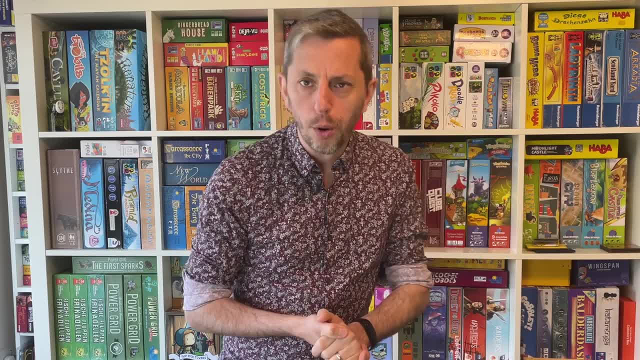 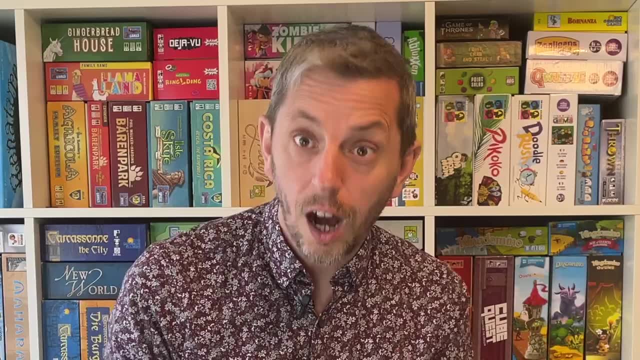 illustrator, the scribblings of an emerging author. Game design is no different to any other art form. When you start out, you do it for the love of it. But crucially, I did do it. My ideas didn't linger in my head. I put pen to paper quickly. 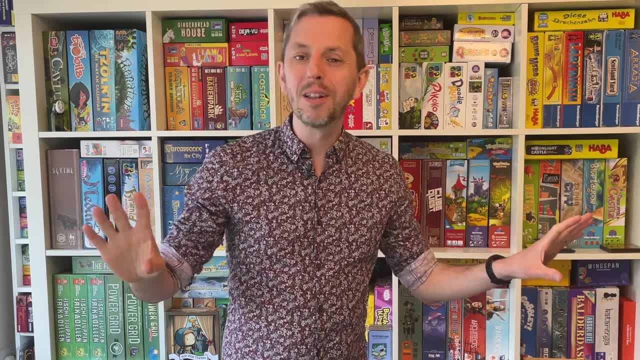 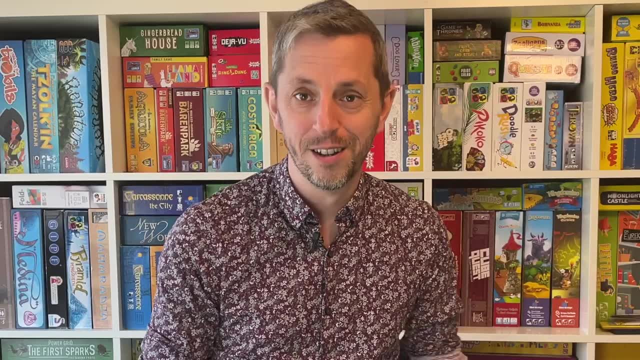 I wasn't embarrassed or fearful. I designed terrible games, but I fixed them as we played. I had no concept of an end result. I only cared about having fun. If you ever meet me in person at a game design meetup, you'll probably find me quiet and polite. 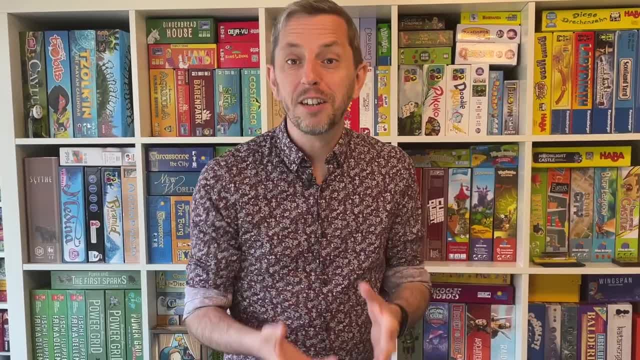 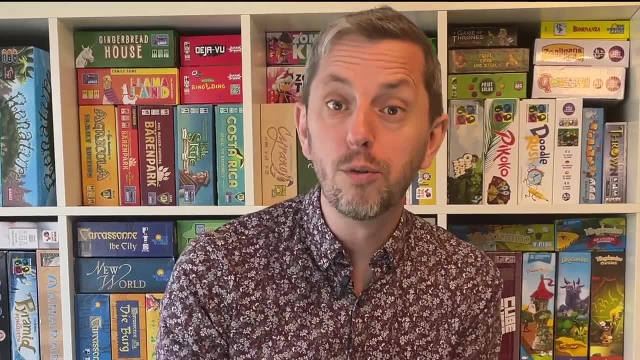 perhaps in a sense of a relationship, but most importantly very friendly. I would love to be a part of society in some way, a little aloof, smug even, and occasionally brash. New designers often try to tell me their ideas and I tend to give them short shrift. I'm not intentionally rude, my mind. 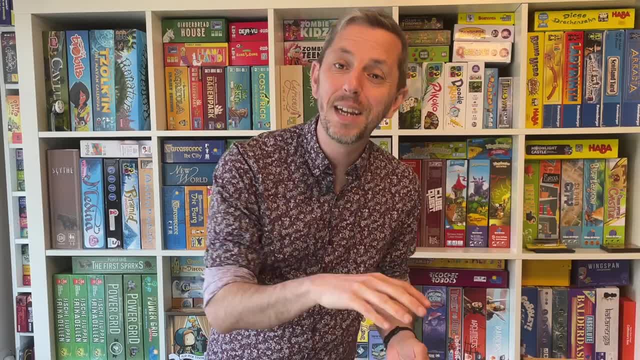 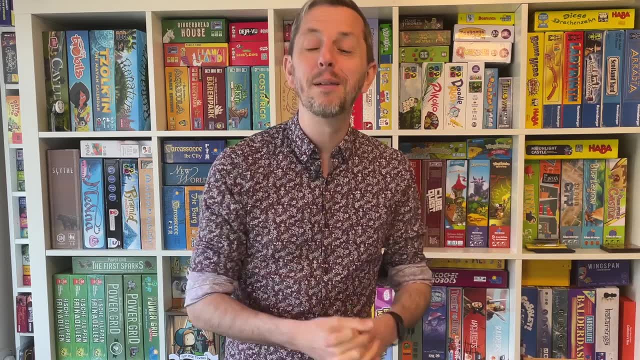 just doesn't work that way. Get those ideas on the table in whatever form they spill out of your muddled mind. Be fearless and unashamed. No one can play the game in your head. Put physical components in front of us and let's take this thing for a spin. Find out all the 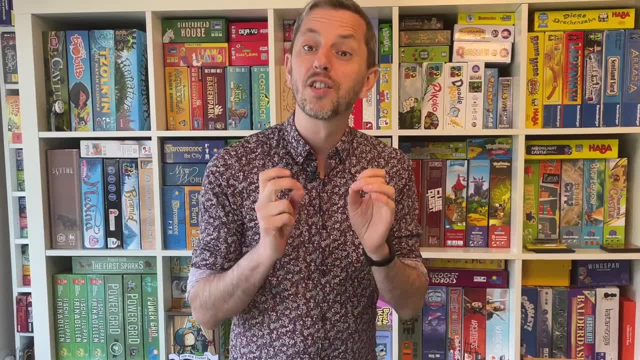 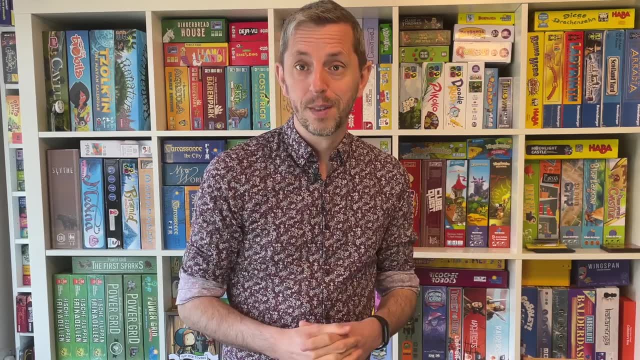 ways it's broken and, most importantly, try to locate the spark, the intangible, non-pinpointable something, the soul of the game, the fun. One of the first titles which really got me hooked on modern games was Dominion, When I started playing over a decade ago there. 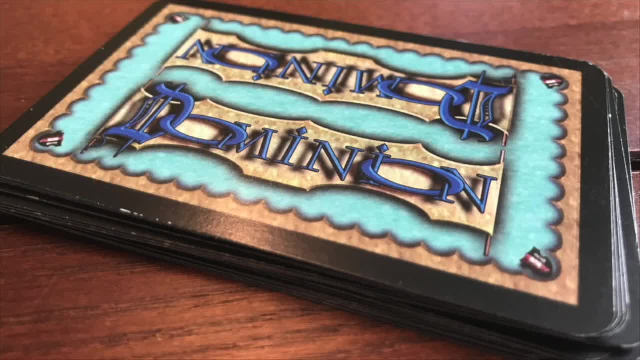 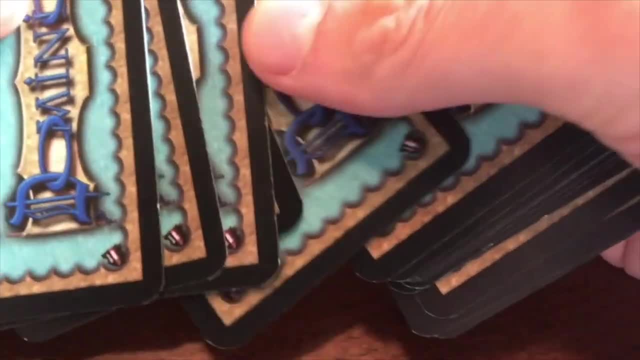 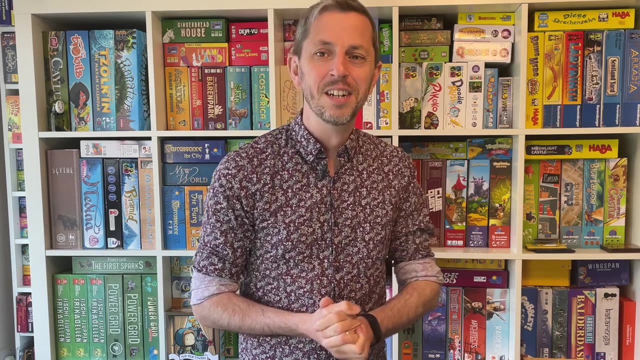 were a couple of expansions available, but there was a thriving community of players creating their own fan-made cards And I quickly threw myself in too, creating wildly unbalanced kingdom cards and forcing games to be unbalanced, Generous friends to suffer their way through frustrating off-kilter sessions. The bulk 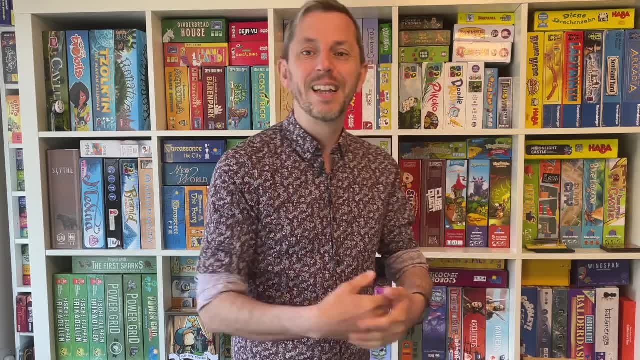 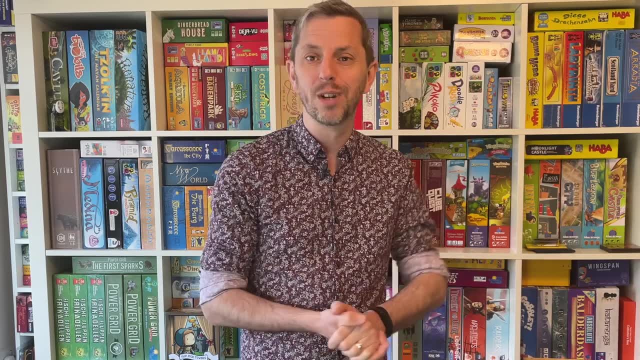 of the fun wasn't playing, it was tinkering: Laying out the cards, tweaking and adapting after each test, Finding images online to blend the cards in with the original game. And it wasn't just Dominion. I recall creating my own expansions for Takenoko, Dicetown and 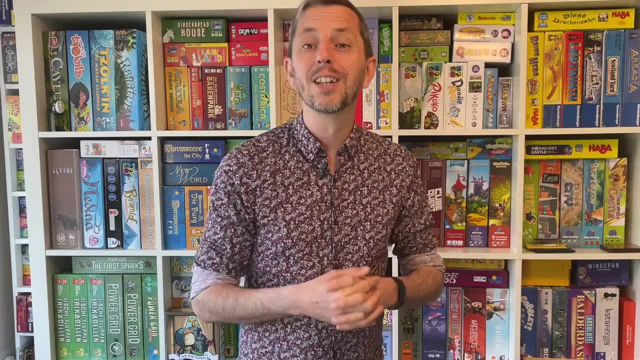 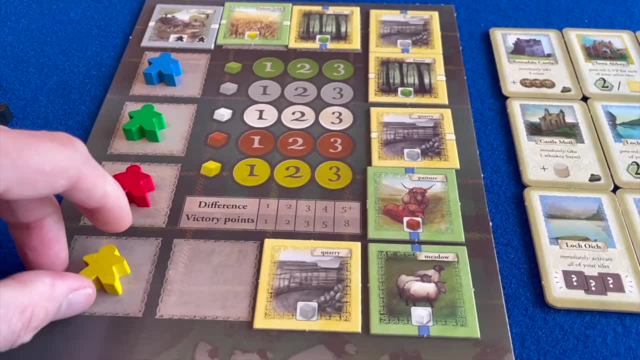 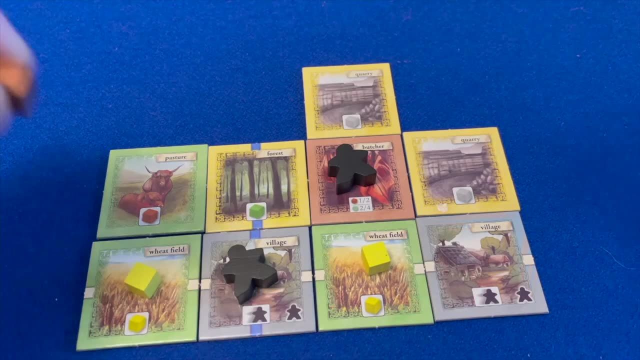 Super Dungeon Explore. My friends must have got fed up of playing ill-conceived variants because before long I found myself creating solo modes. I remember playing a lot of Glenmore and Drumroll by my own solitaire rulesets. This is a great way to learn about board game design with a very low barrier to entry. 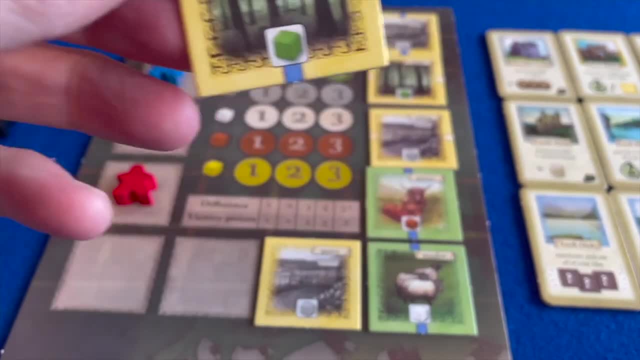 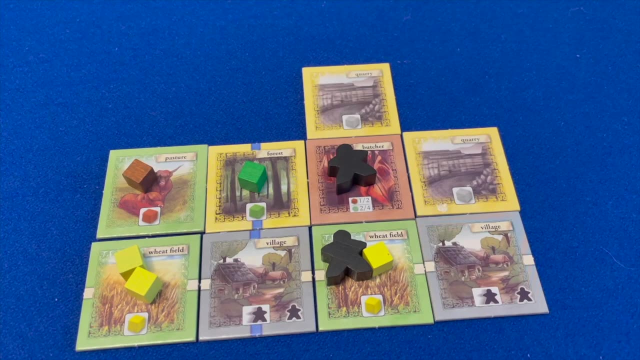 The game already works. You've got a sound system, a fully realised world. When you tweak such a game, bolt bits on or chop bits out, you start to understand the interwoven mechanisms at play and how a seemingly minor element of gameplay functions as part of a greater. 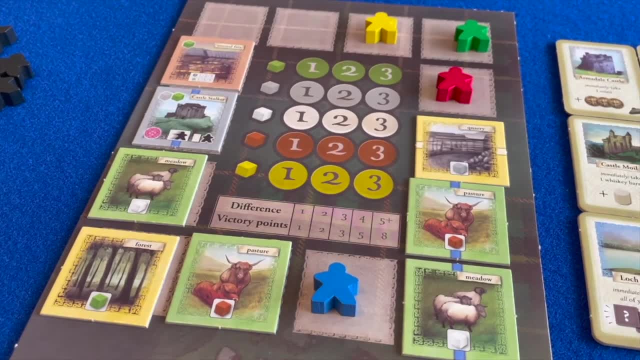 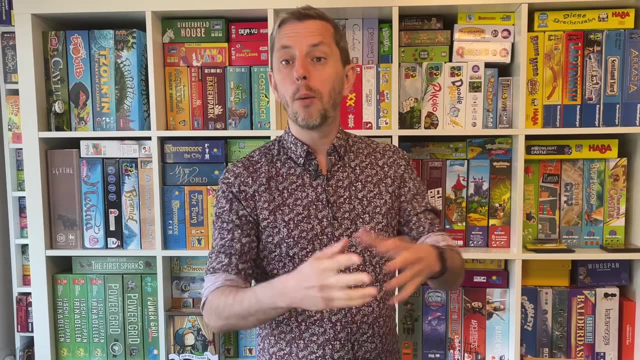 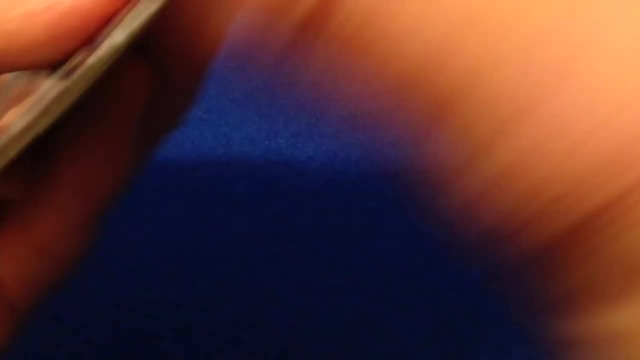 whole. In game design, every aspect has been carefully considered and if it made the final cut, it's there for a reason. What happens if you lop that bit off? How is the experience altered for the players? It's a great exercise for a game creator learning their craft. What happens in Dominion? 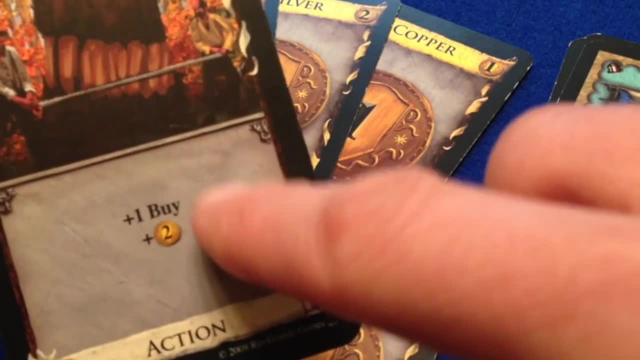 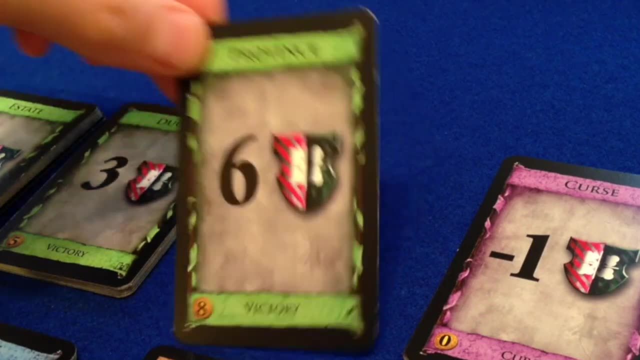 if you shuffle all the cards together and reveal a market of 10 random cards. instead of using predetermined decks, Why aren't purchased cards placed on top of your deck for immediate use instead of the discard pile? Well, try it and you might find out. 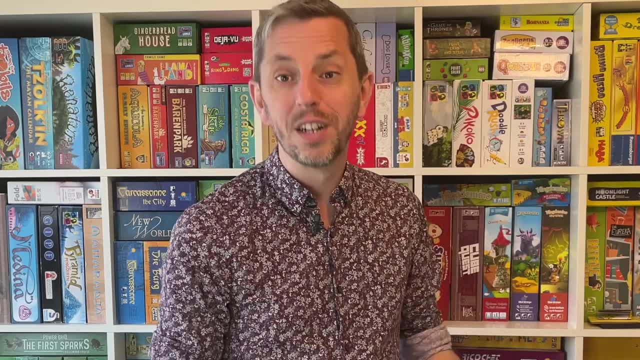 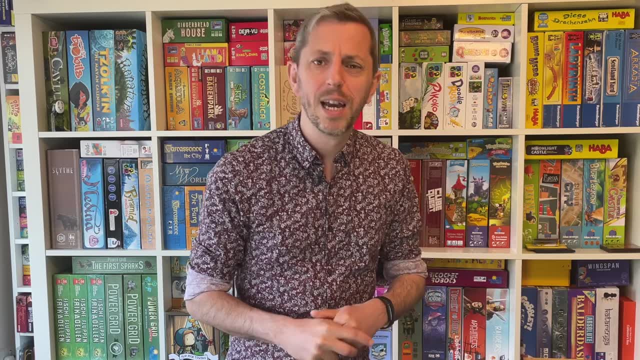 Ten years ago, if I wasn't playing games, I was tweaking them and I still didn't consider myself a designer. One week, on games night, a friend arrived with a prototype game he'd put together. It was an area control game about fish populating a coral reef. This was the first time I'd 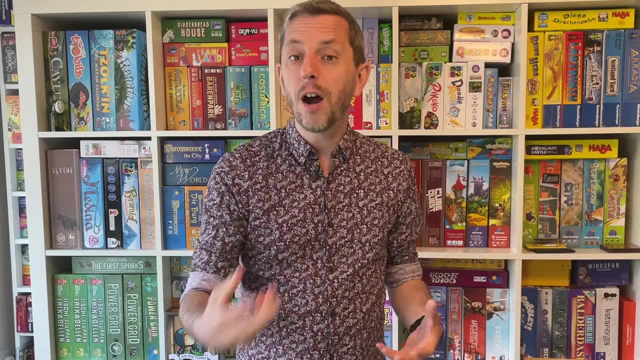 played a game which was hugely imaginative and promising, vibrant and joyful, but also gloriously, deliciously broken Muscle memory from 30 years of playing games. It was the first time I'd played a game which was hugely imaginative and promising, vibrant and joyful. 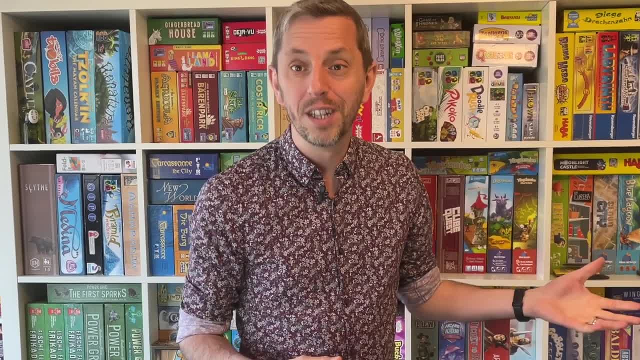 but also gloriously, deliciously broken. Muscle memory from 30 years of playing games. It was the first time I'd played a game which was hugely imaginative and promising, vibrant and joyful, but also gloriously, deliciously broken. Three decades of game design, though I'd never called it. that kicked in and I became 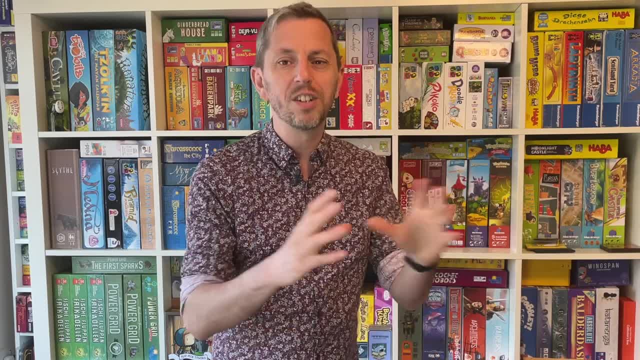 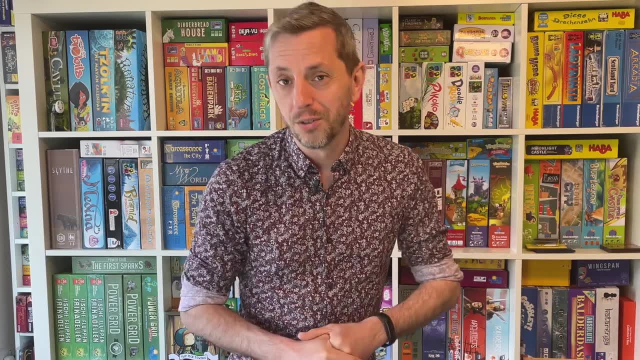 obsessed with this thing. I was the worst sort of playtester. I wanted to change everything and I bombarded my friend with praise, criticism, helpful suggestions and unwelcome alterations. After several weeks of politely incorporating elements of my feedback into the game, my 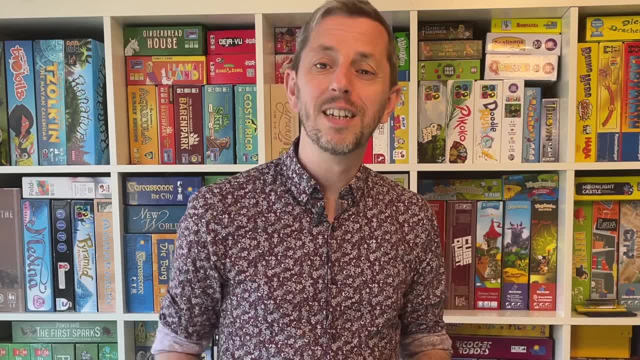 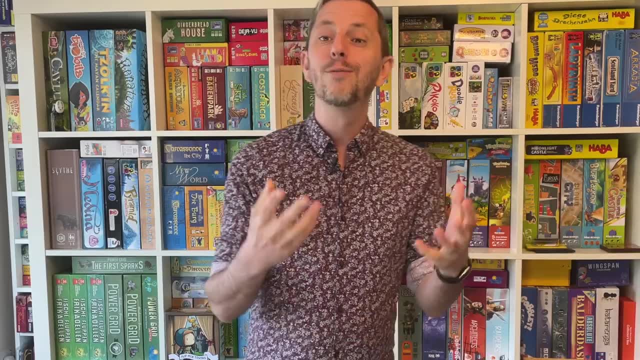 designer pal gently suggested that I take all my ideas and make my own game, leaving him to develop his coral reef project in the manner that he deemed fit. I had developed a passion for design and I wanted to do more, but I had never created. 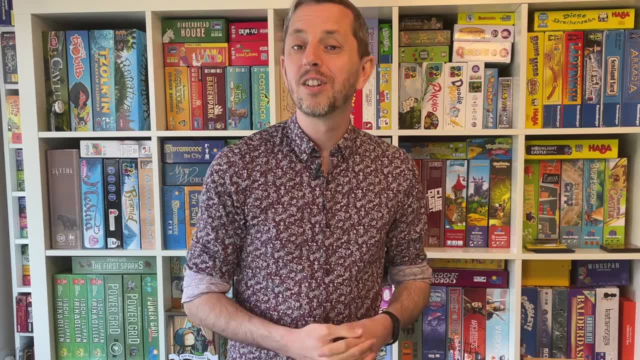 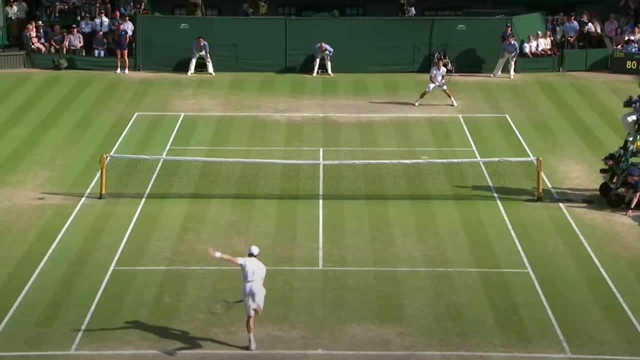 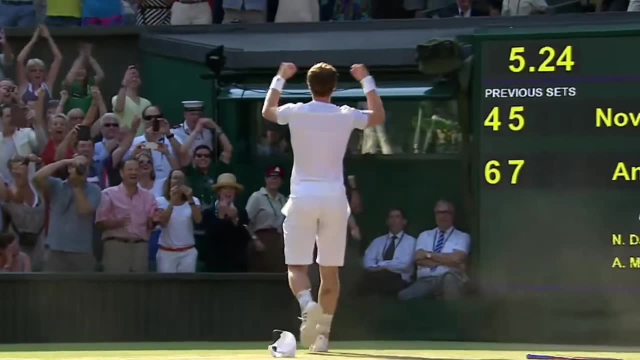 a new world from scratch. All of my design experience to date was based on tweaking and developing existing rulesets. In 2013, I was watching Wimbledon. Andy Murray was promising to end a 77-year wait for a Brit to claim the men's singles title, and I thought to. 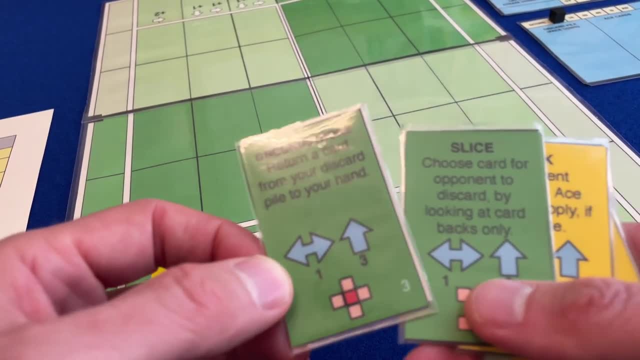 myself: if I don't have my own ruleset, why don't I just adapt an existing ruleset, such as tennis, into my own ruleset? I thought to myself: if I don't have my own ruleset, why don't I just adapt an existing ruleset, such as tennis, into my own ruleset? and I 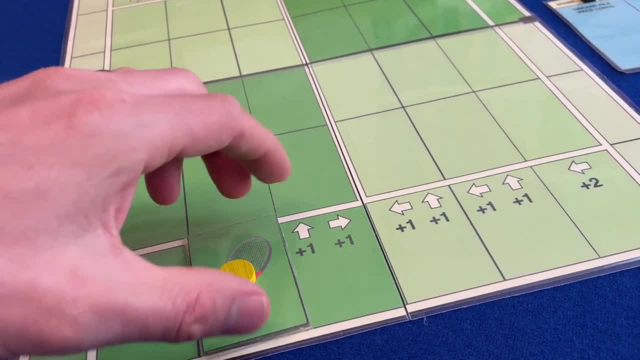 thought to myself: if I don't have my own ruleset, why don't I just adapt an existing ruleset, such as tennis, into a board game? How would that work? This is my prototype for Advantage Tennis, a project I briefly shared online as a print. 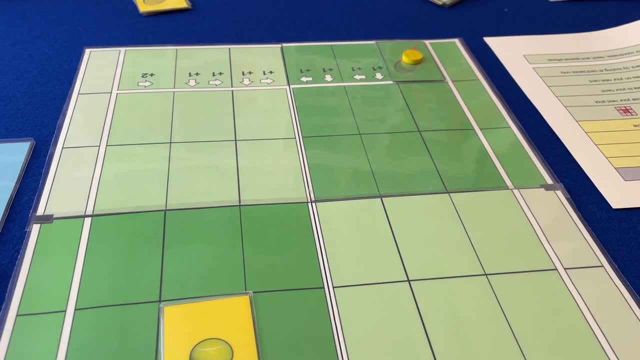 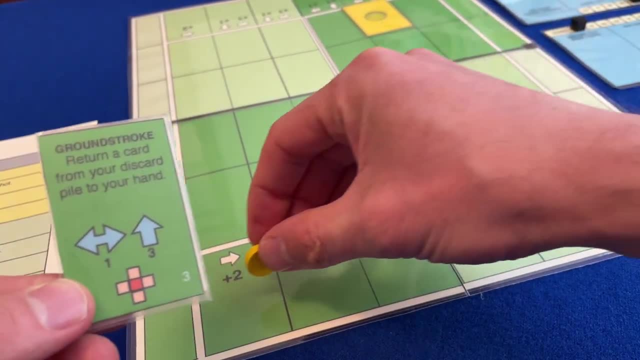 and play game, along with two related games using similar mechanisms: Advantage Cricket and Advantage Baseball. Advantage Tennis is a simultaneous card selection game in which players try to deduce where their opponent is going to land the ball and then successfully return it. It's not a good game. 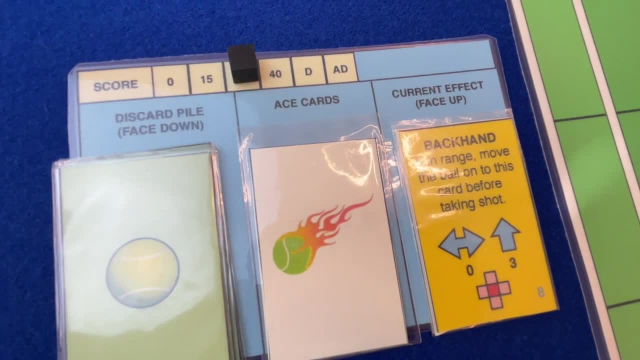 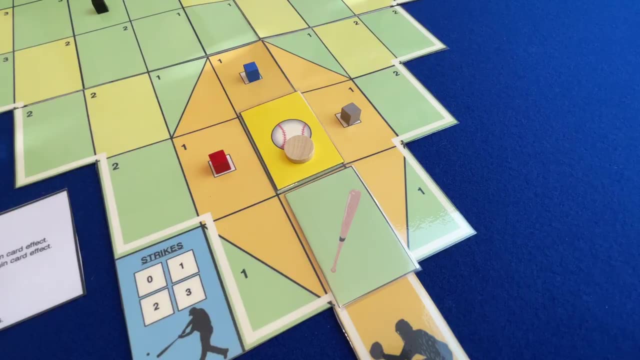 But this was the first time I genuinely considered myself a designer. I foolishly created listings, the Board Game Geek database, to share files for these three print and play games, A decision I regret And despite many requests over the years, I can't get Board Game Geek to remove the pages. 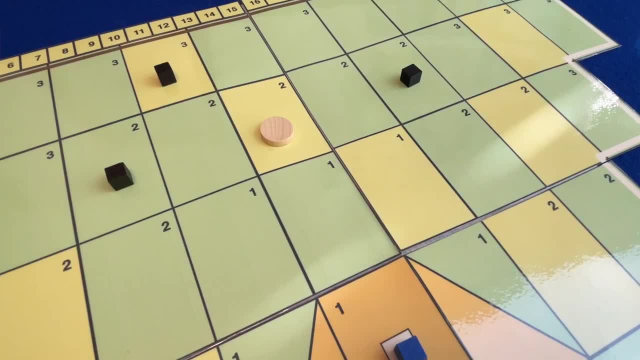 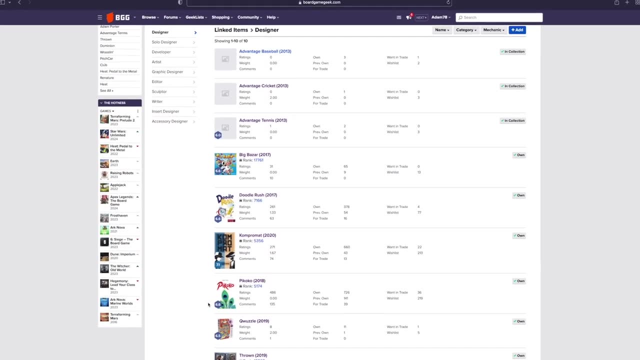 and, frankly, they don't belong there. These weren't polished games, they were early prototypes. BGG functions a lot like a CV for a professional game designer As of the spring of 2023. I currently have eight published games to my name, and I'd rather that these precursors didn't muddy the. 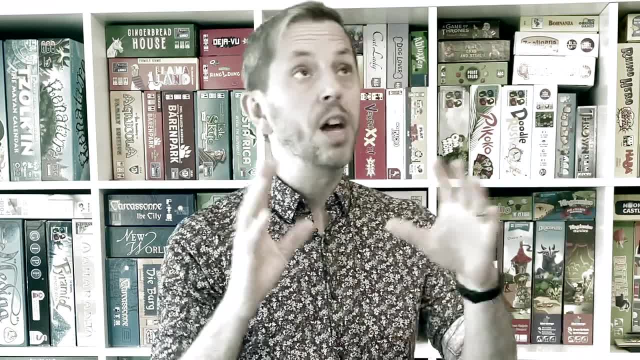 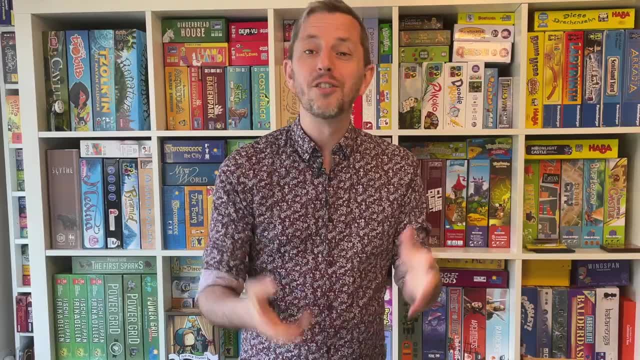 picture. So there's a lesson for you first-time designers out there: Don't create a Board Game Geek page for your game unless it's on the cusp of being published. You might regret it later. I enjoyed creating these three games so much I wanted to do more. Now I'm not really a big 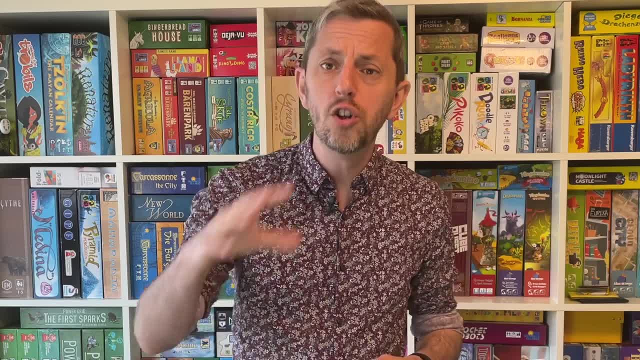 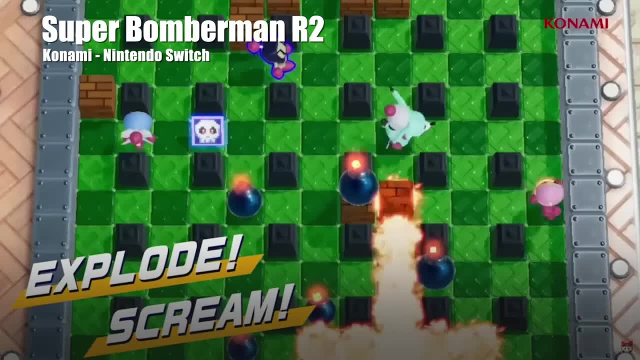 sports fan, but I was still fearful of creating a wholly new rule set from scratch, So I went looking for another pre-existing set of rules to adapt. My next design project was recreating my favourite video game, Super Bomberman, as a board game. 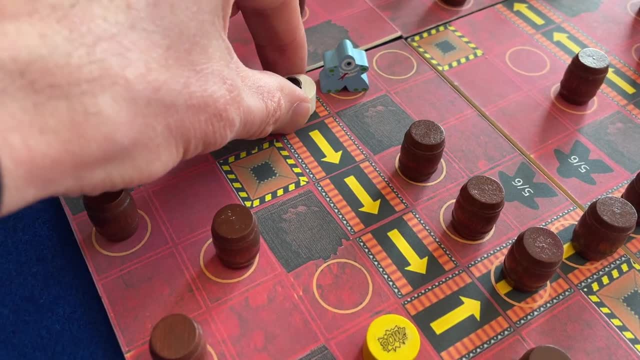 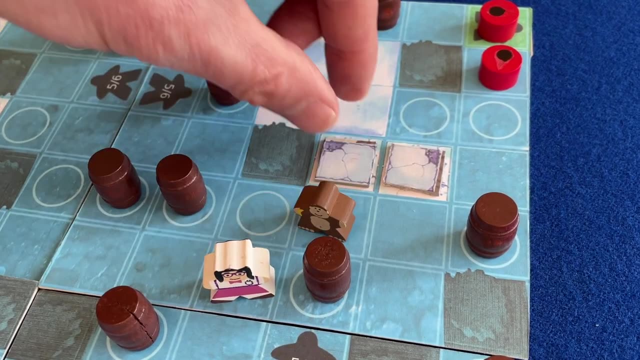 I went all in on this one. I spent weeks laying out the artwork, creating variable arenas, buying wooden components and recreating every aspect of the original game, with vague daydreams of publication and in the knowledge that I would never be able to get the license to the video game. 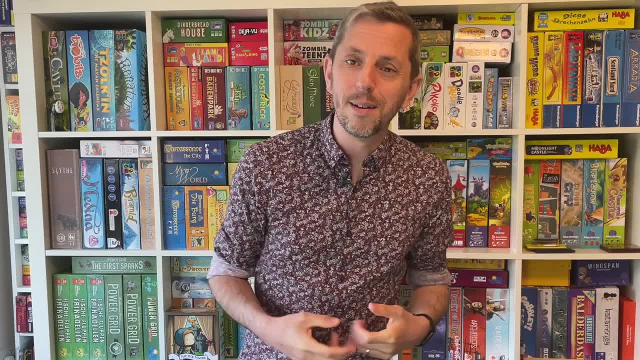 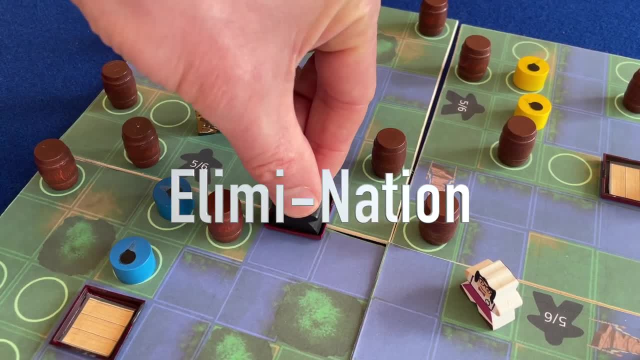 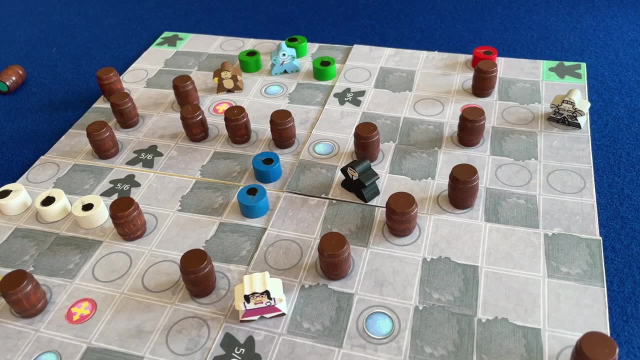 characters. I devised my own narrative: A Hunger Games or Running Man styled arena full of wacky combatants. I called the game ElimiNation. ElimiNation was a fully realised game. It functions well and it simulates most of the mechanisms of the video game, While Bomberman is played in real 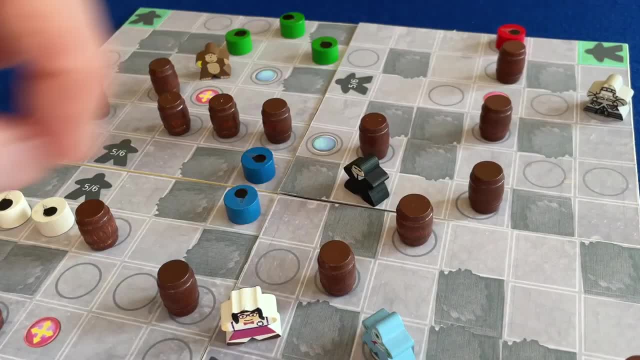 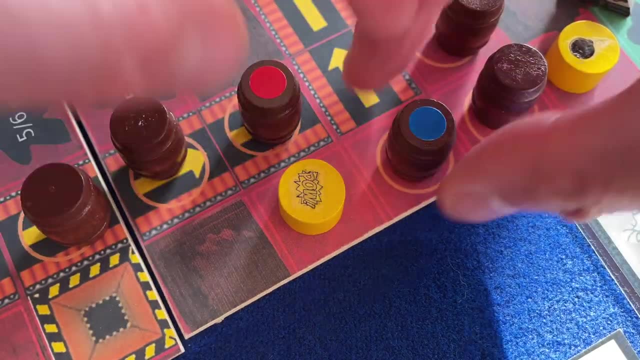 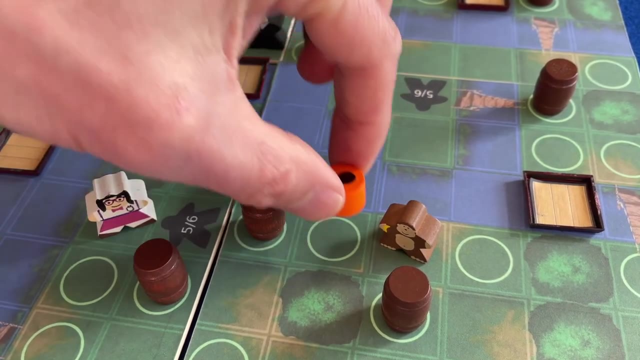 time. ElimiNation is turn based and it uses an action point system, That is to say, players have a number of action points available each turn, which can be spent to do a variety of things: Move a space, drop, kick or throw a bomb. Popular in the early 2000s, action point games are: 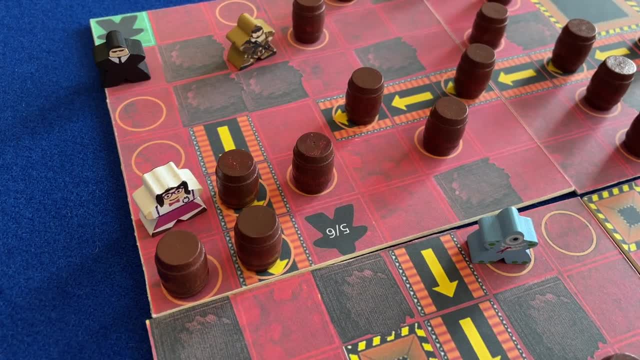 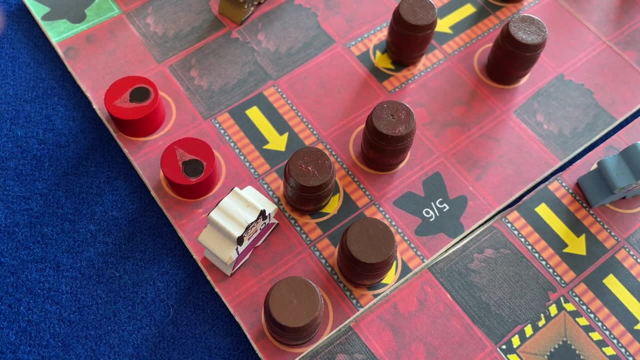 notorious for creating an arduous experience. Players are often paralysed as they weigh up the massive number of choices they have to make. It's a game where you have to make a choice between one of the two. The one element of Bomberman that ElimiNation failed to recreate was the speed of. 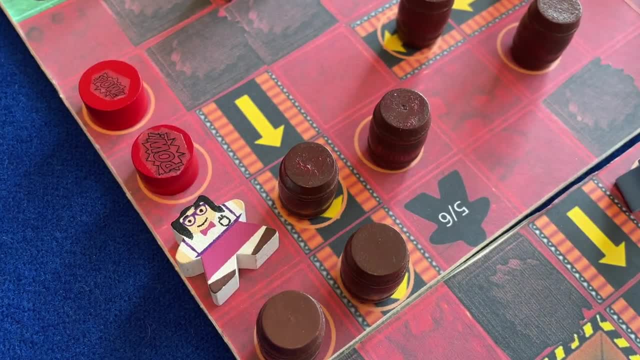 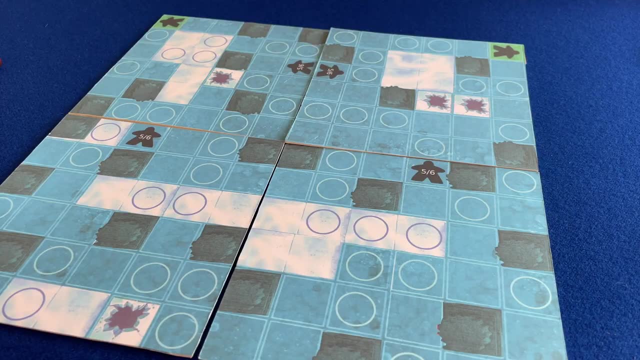 play, arguably the defining feature of the original game. If you ask a group of designers about using artwork in early prototypes, they will tell you to avoid beautifying your game because you'll be adapting, destroying and recreating it often and wasted hours spent laying out graphics not to 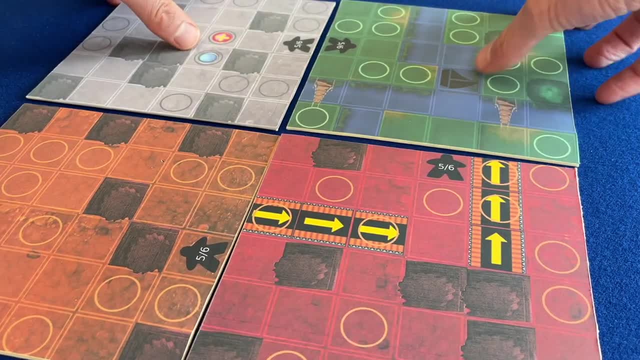 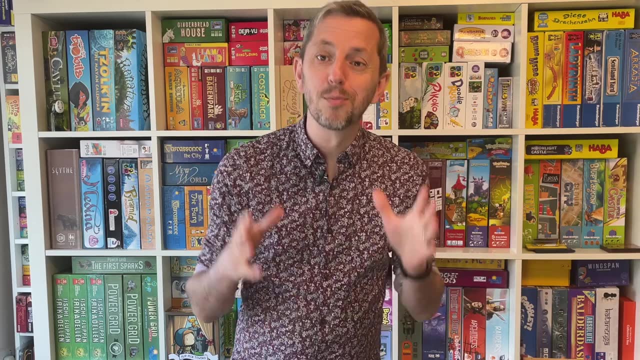 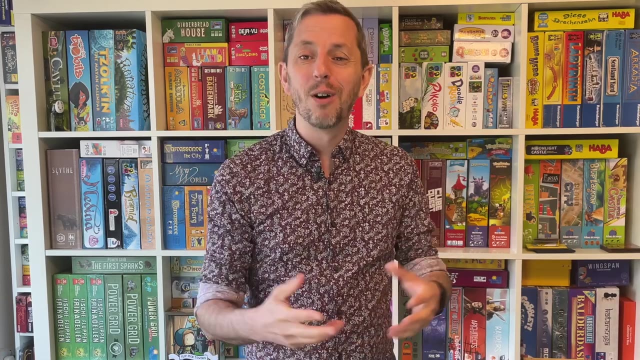 mention the cost of ink will make you reluctant to carry out necessary changes. I must admit I differ from most on this point. Laying out the artwork for a prototype is one of the most enjoyable parts. I get lost in it. hours pass by in the blink of an eye. The process of laying out 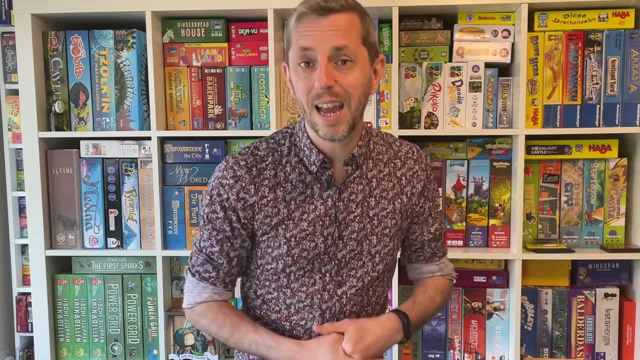 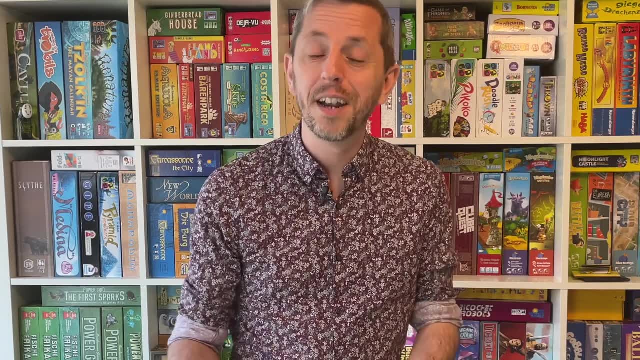 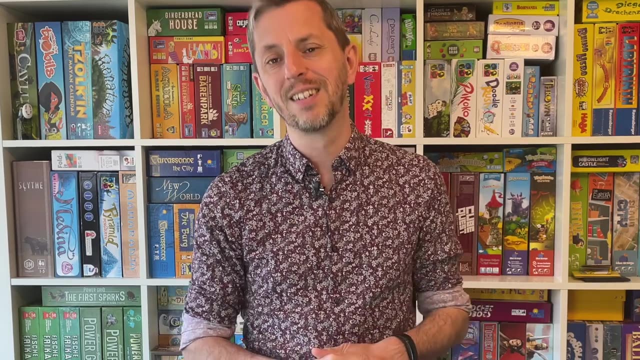 artwork, even as a placeholder, helps me to fall in love with the game, And frequently time spent in this focused creative mode helps me identify answers to mechanical issues, as if from nowhere, a solution will pop into my brain. addressing an issue identified in a recent playtest I cherish. 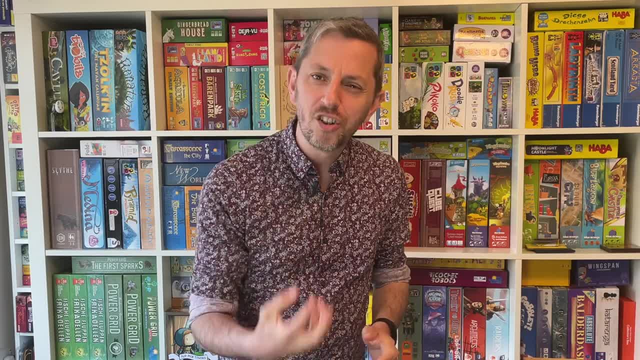 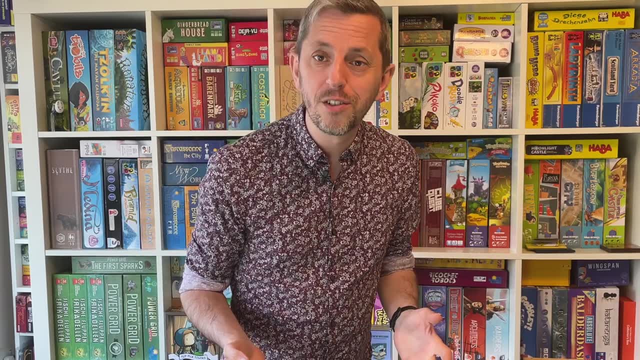 these hours laying out graphics and imagining what the game could become. If you're designing for pleasure and simply want to create a wonderful game to play with friends or family, with no aspirations to publication or commercial success, I fully support designers going all in on their 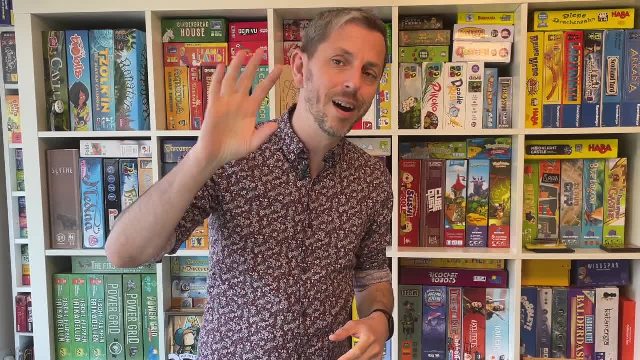 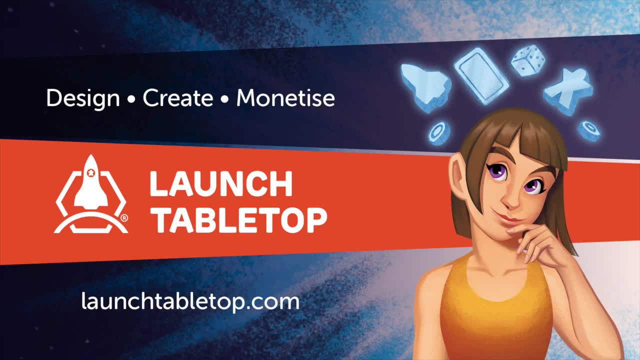 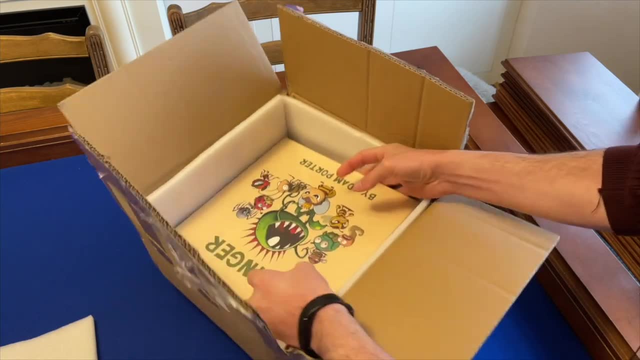 project. Immerse yourself as deeply as you like. Create beautiful prototypes. One way of doing this is to use Launch Lab, a print-on-demand service from Launch Tabletop. the sponsors of this video, Launch Tabletop, are a full-scale board game manufacturer, so games produced through their 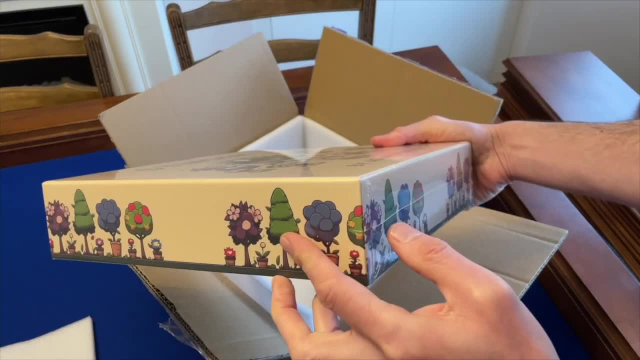 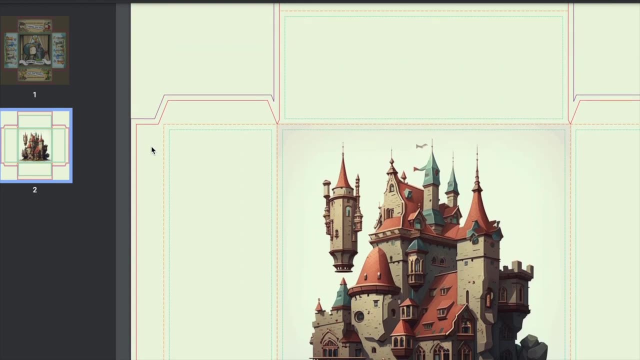 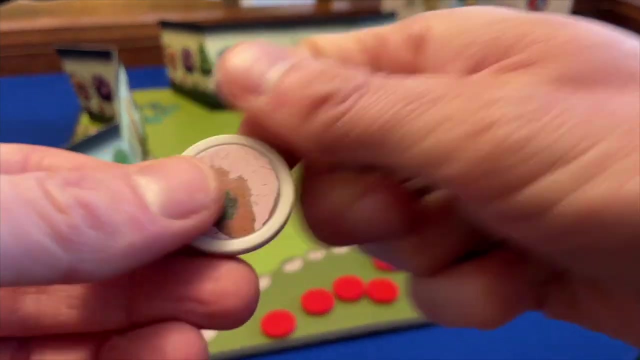 Launch Lab service are indistinguishable from a professional project. You simply create an account, select your components and download templates to lay out your artwork in the correct configuration. The games will be posted to you wherever you're located in the world in an impressively short timeframe at a very reasonable price. 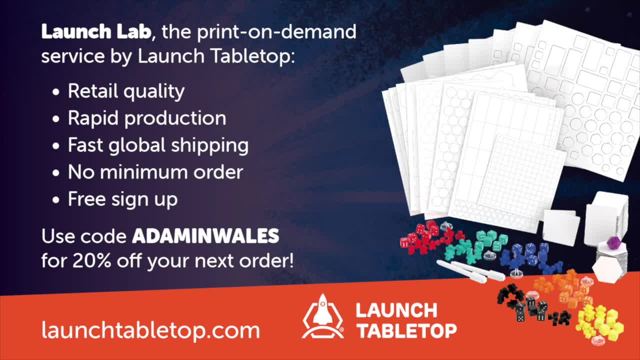 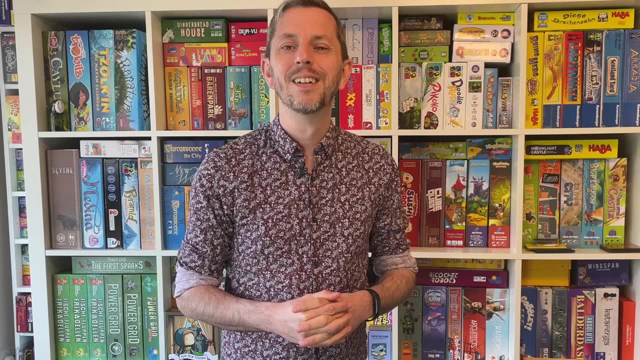 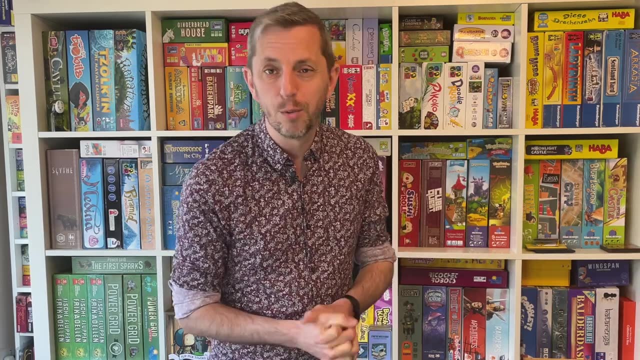 If you fancy creating a high-quality prototype, visit launch-tabletopcom, upload your files and use the code. I was fortunate that around the time I really started to indulge my new passion for design, a regular designer meet-up was advertised by Rob Fisher, a local game inventor who had self-published. 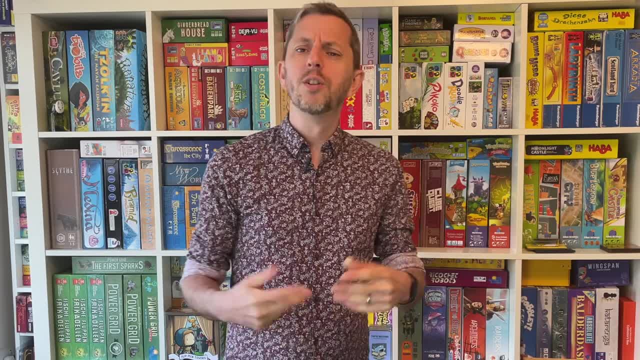 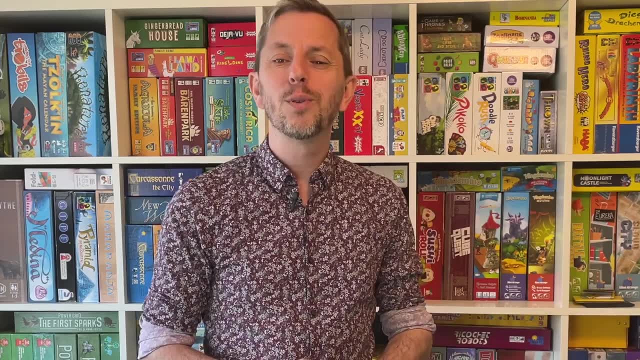 his first game a couple of years earlier. I attended the inaugural meeting for the Cardiff Playtest Group back in 2014, and my professional game design journey began. Surrounding yourself with other game designers is inspiring, informing, challenging and rewarding. 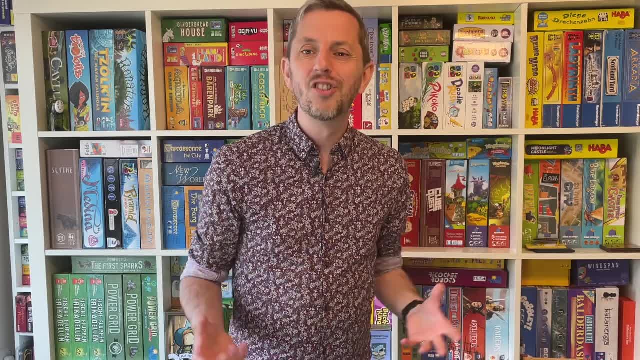 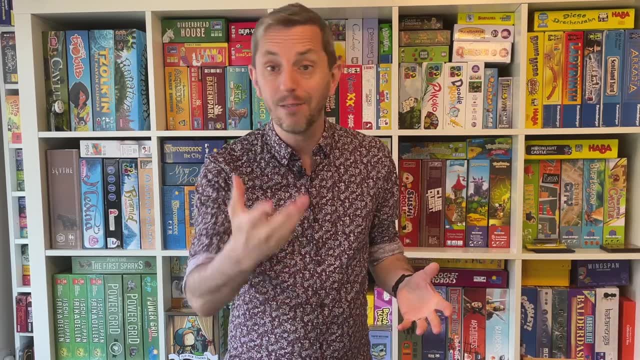 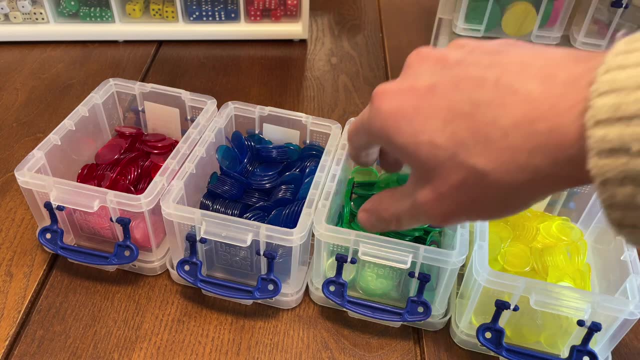 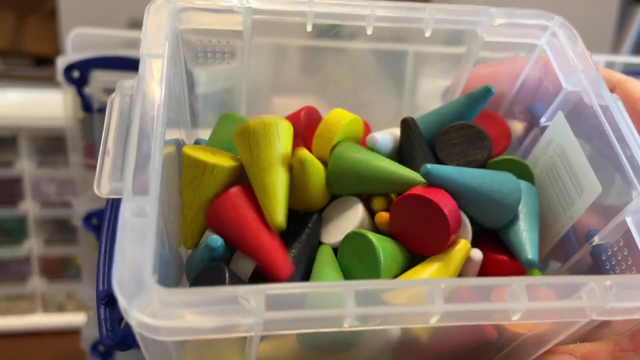 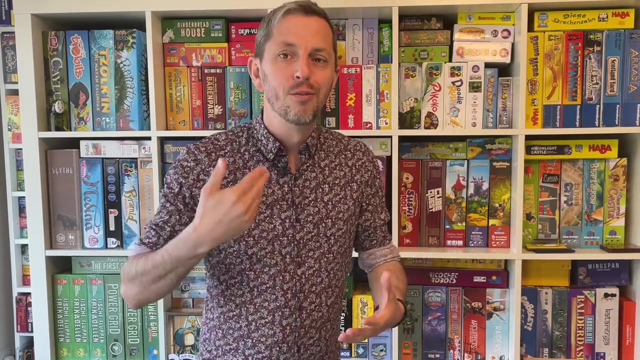 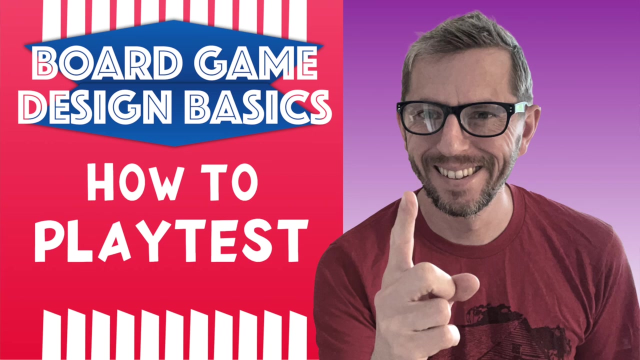 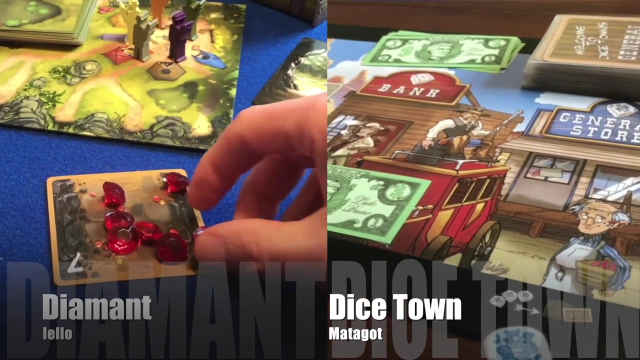 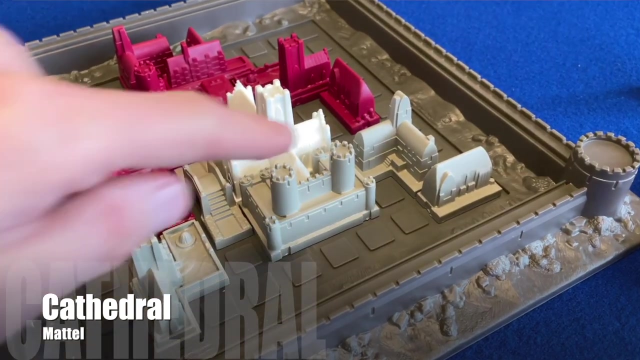 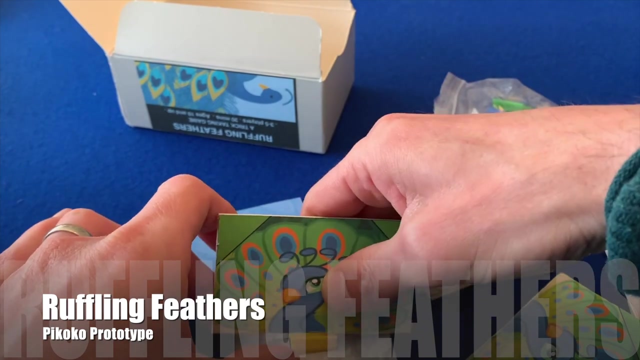 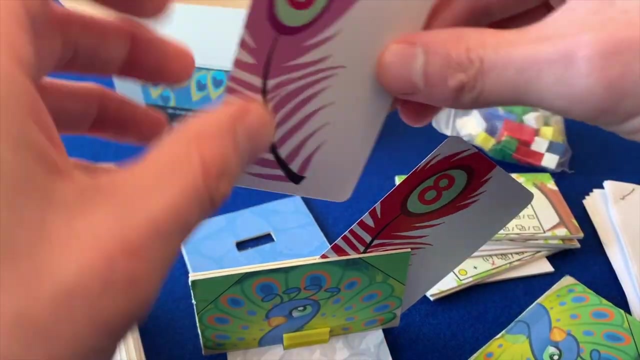 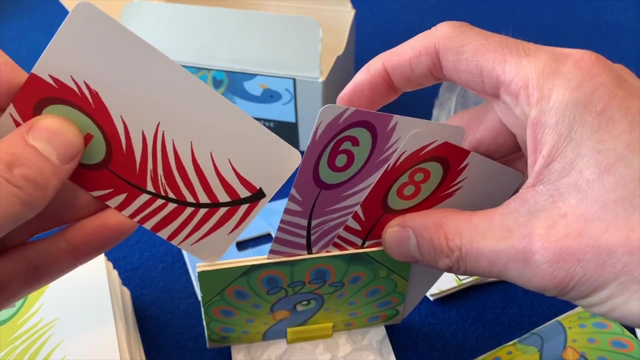 I hope you've enjoyed this video and I hope you've enjoyed the rest of the video. Thank you so much for watching and I'll see you in the next one. Subtitles by the Amaraorg community. This video has turned into a potted history of my own early experiences as a game designer. 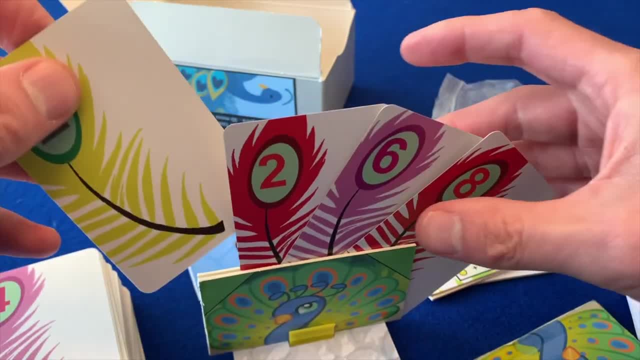 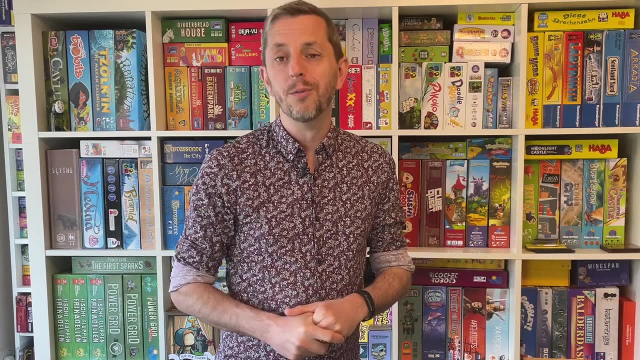 and I'm not sure it could be any other way. This part of the process is so personal I can't speak for others, but hopefully there are lessons here which help you with your own journey. There are some pieces of advice which are so frequently cited by game designers in playtest. 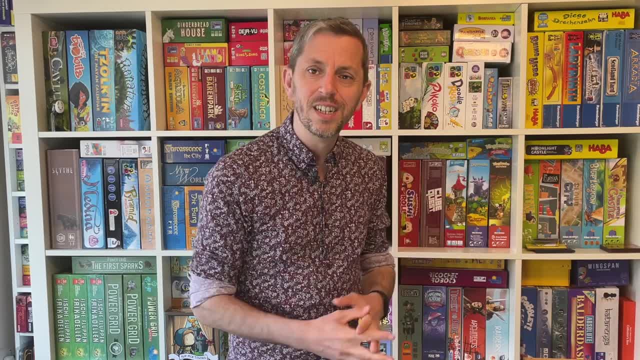 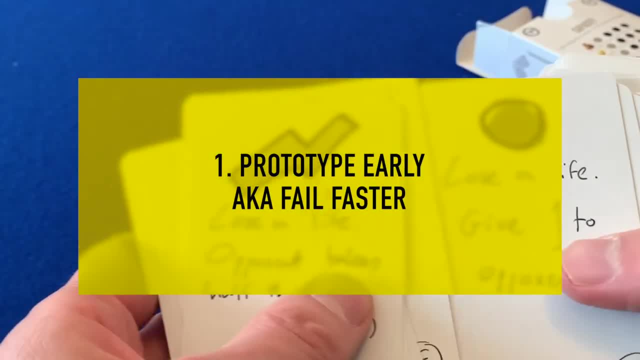 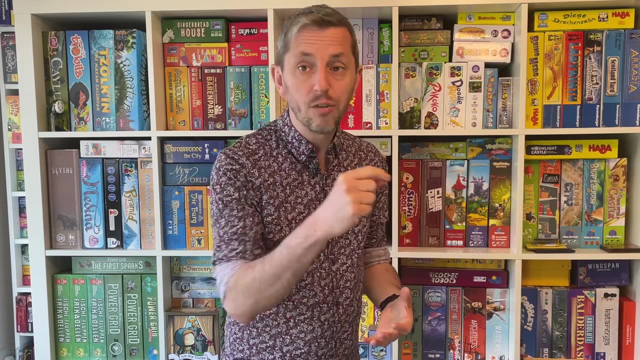 groups and online forums and stated with such certainty that I'm not the only one who has had to revisit and critique them. Number one: Prototype early, Sometimes phrased as fail faster. The frequent advice to prototype early is sound: Get your ideas out of your head and onto the. 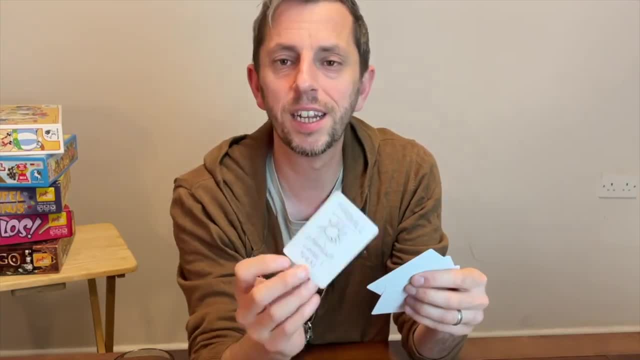 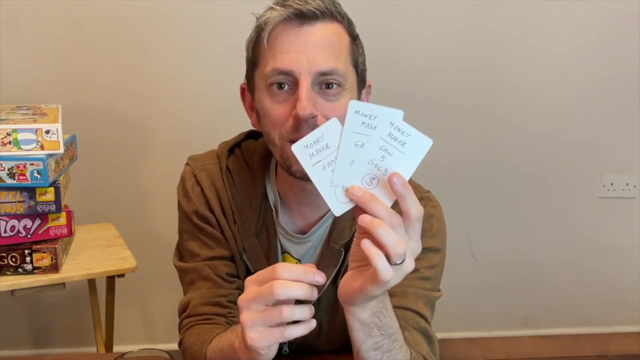 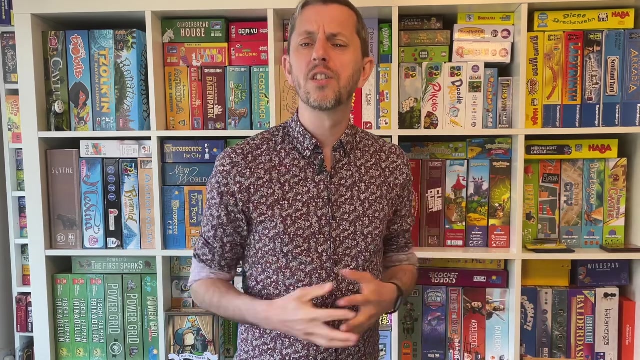 table before they become corrupted, cross-contaminated and weird. A physical prototype is a constraint. It reigns you in and contains your ideas, grounding them in reality. A new game designer once told me that he had no need of playtesters: He could run simulations of all of the various game states and 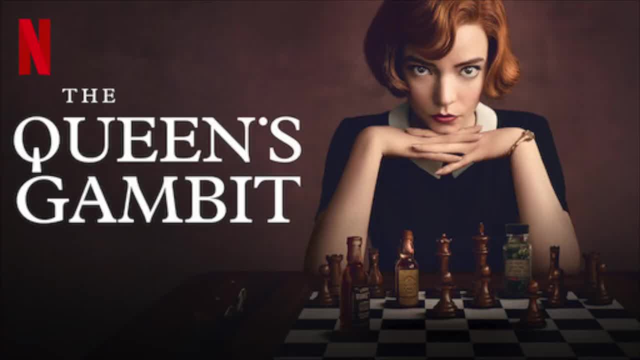 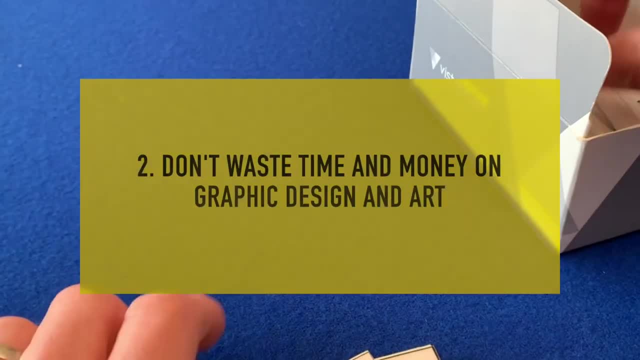 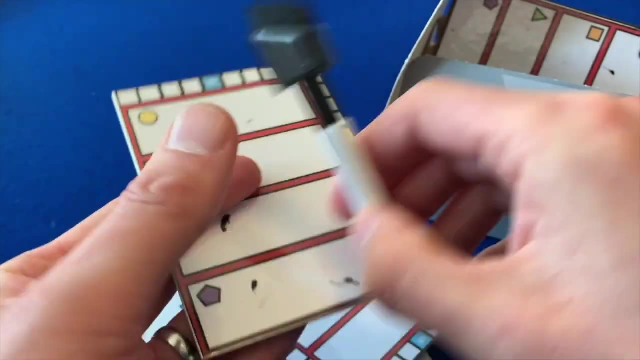 scenarios in his head, like that girl from The Queen's Gambit. This is nonsense. You're not ChatGPT. Get it on the table. Don't waste time and money on graphic design and art. The frequent advice to keep your prototypes cheap and ugly is also sound if you're aiming. 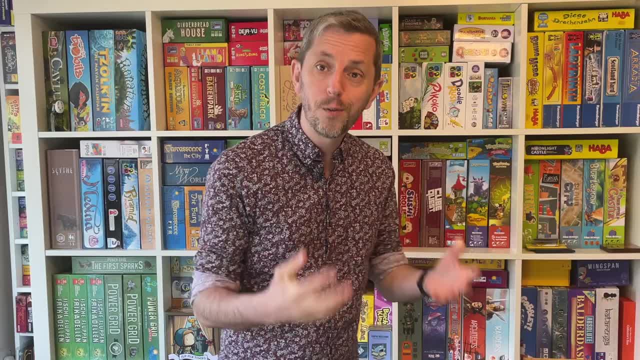 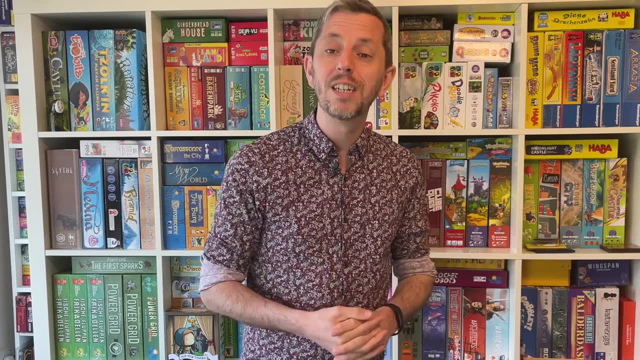 to streamline the process and reduce costs. But if you find joy and inspiration immersing yourself to totally in a design project and you're willing to accept the extra time and money this approach costs, then I say go for it. Number three: Don't base your 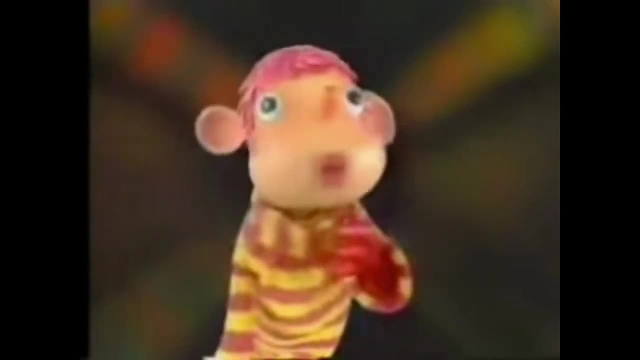 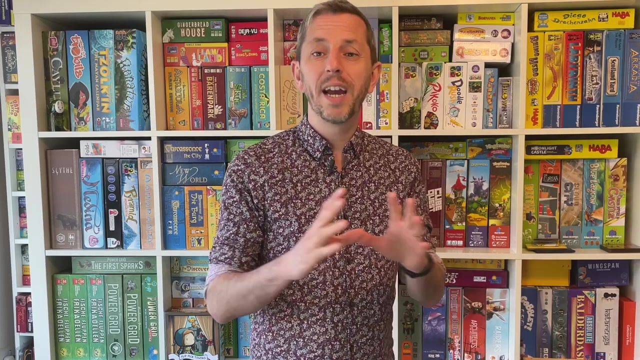 game on popular properties from film or TV. Well, this advice is essential if you're hoping to publish your game. Most publishers don't want to invest in licensing rights and your Ted Lasso football game is going to scare them off, But in the early stages. 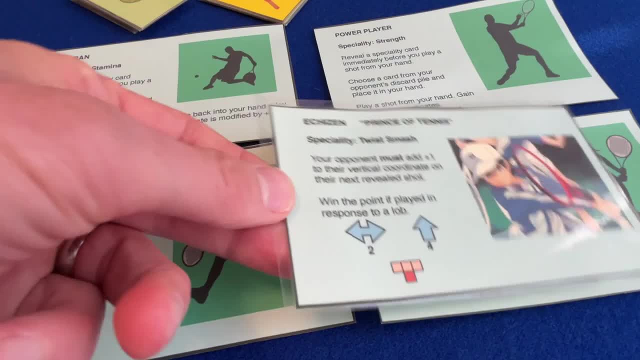 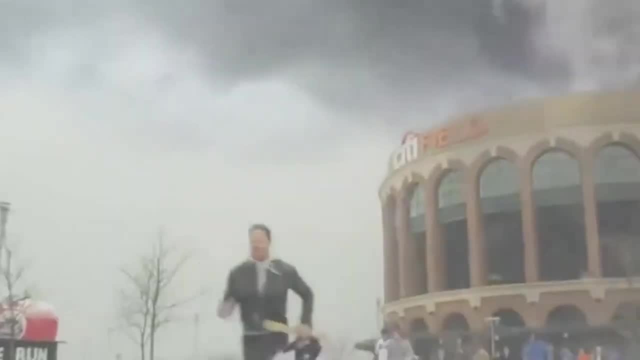 of experimenting with design. I think this advice is limiting: Rip off anything and anybody, I say just as long as you're not planning to sell anything. You're educating yourself and fully realised worlds from popular intellectual properties might give you the inspiration you need. 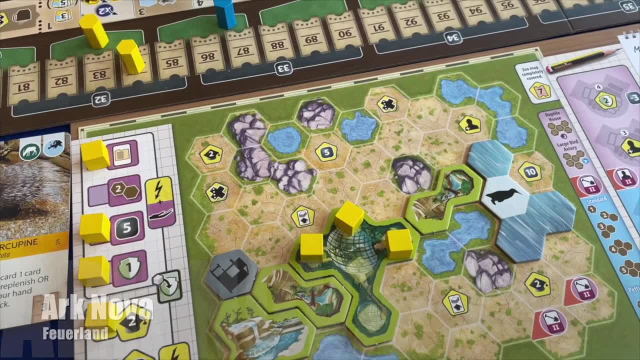 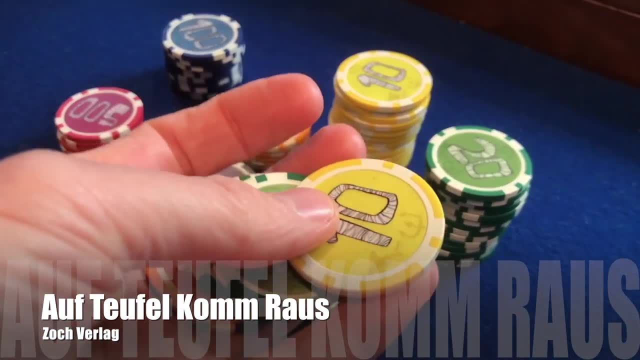 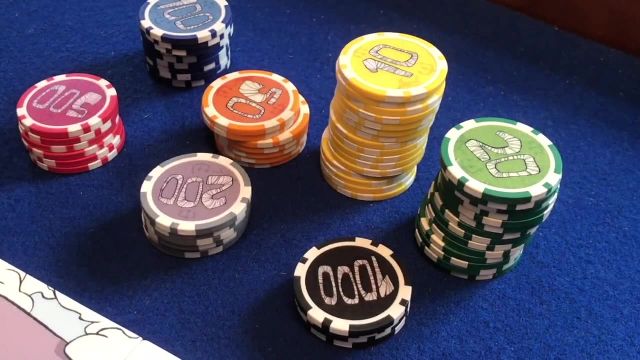 Number four: Play many games, Absolutely. This is going to inspire you. Many of the problems you hit when designing your own games will have been encountered by designers before you and overcome. There's no need for you to repeat those struggles. Play loads of games and fill your designer toolbox. 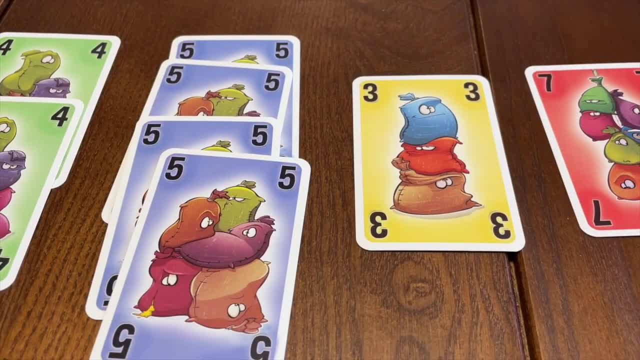 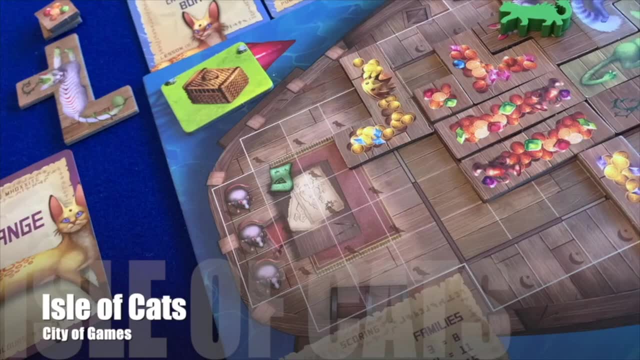 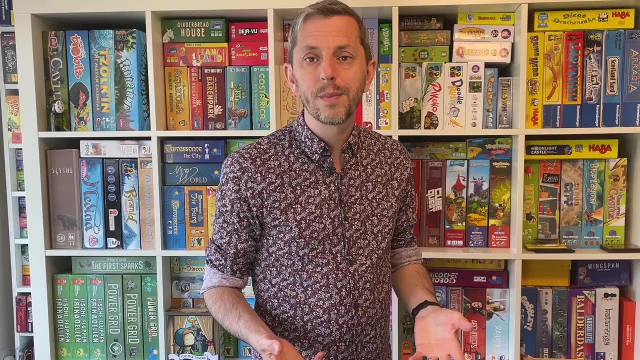 with mechanization. Don't let budget stand in your way here. If you're designing for publication, you need to be up-to-date, playing the latest games. But most games will have regular gaming meetups where you can play a variety of games without having to spend a penny. 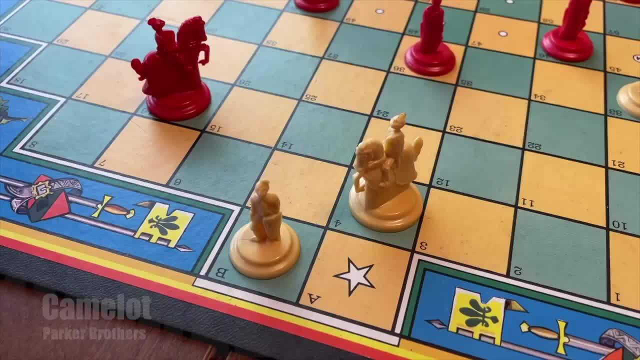 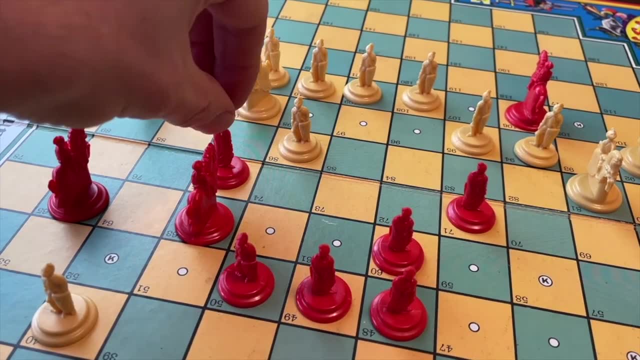 If you're designing for pleasure, well then, it doesn't matter how up-to-date you are. Pick up any old game from the back of your closet or from the dusty shelves of a charity shop, But you must play regularly to stay inspired. 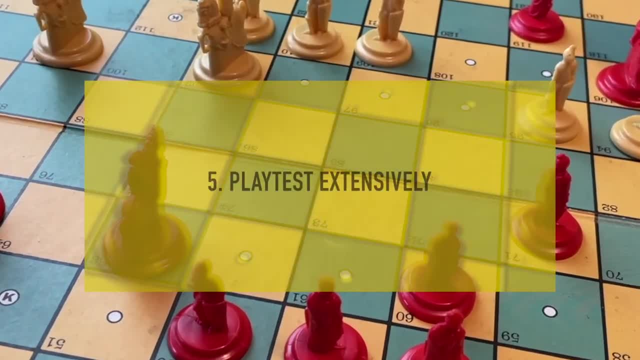 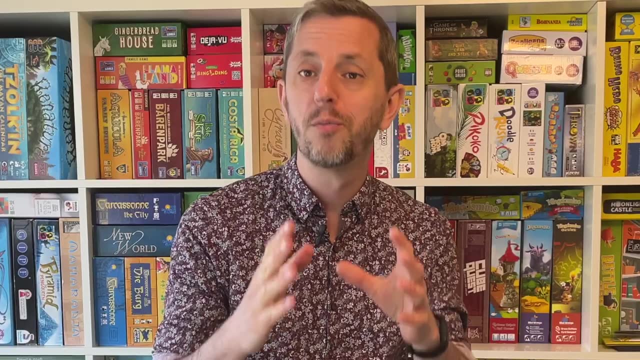 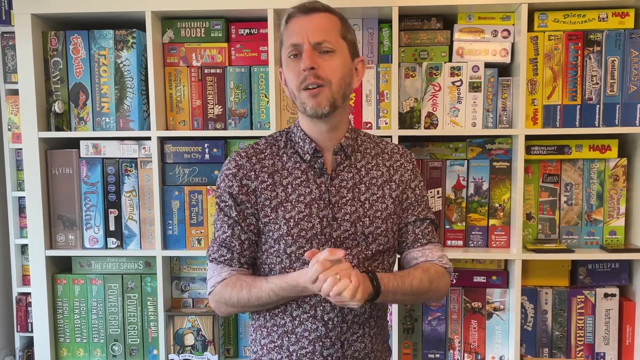 to keep those creative cogs turning. Number five: Playtest extensively. Well, this is crucial for a professional designer. It's optional for an amateur. You can playtest as much or as little as you like. Lots of playtests are going to teach you a ton about design. 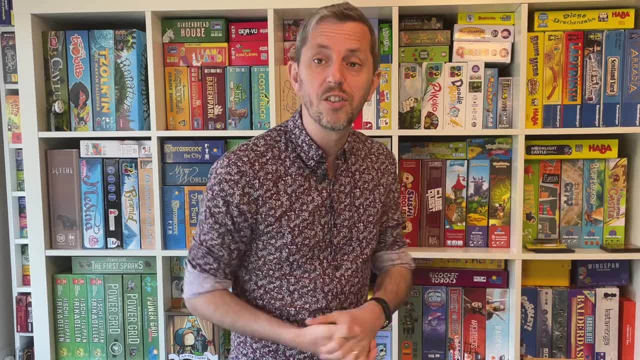 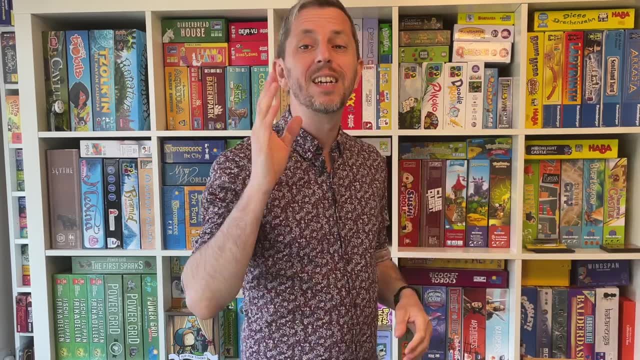 but if the lack of a playtest group is a barrier preventing you from realising your vision, make it anyway. Creating a broken, unbalanced game is still an achievement, and I'd rather it existed than in your frontal lobe. Just don't try and sell it to me. 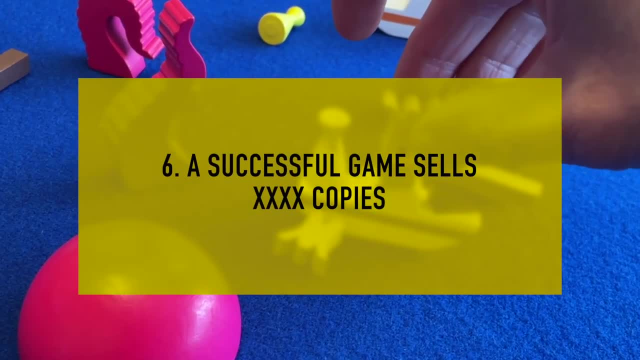 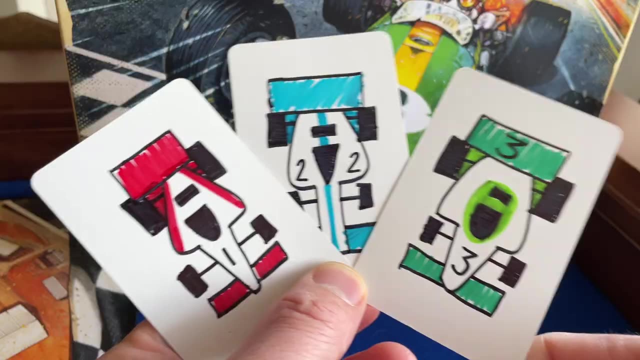 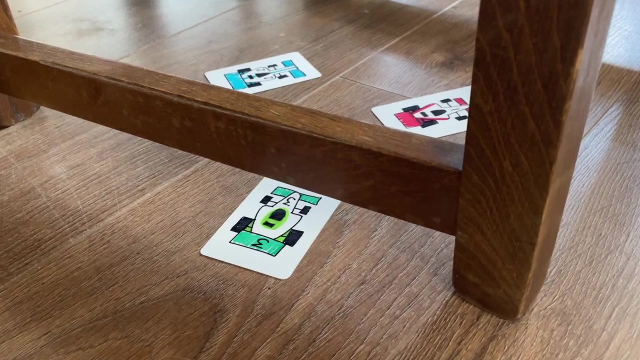 Number six: A successful game sells xxxx copies. Well, this is short-sighted. You define success as you see fit. When I was a kid, success meant facilitating an enjoyable afternoon flicking cards around the coffee table with my mates. A decade ago, success meant faithfully recreating. 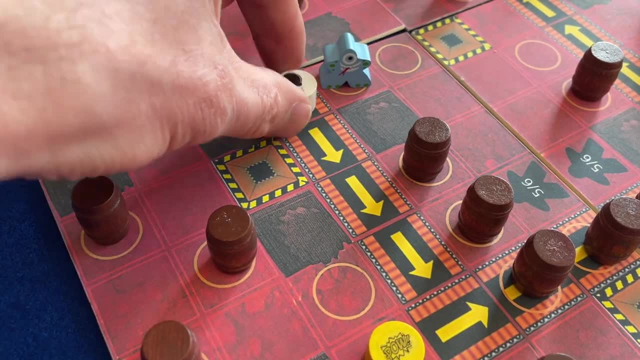 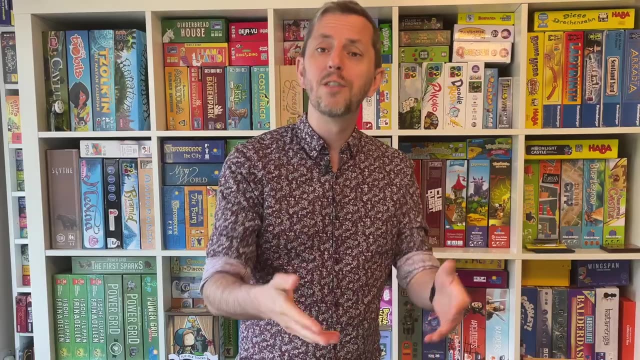 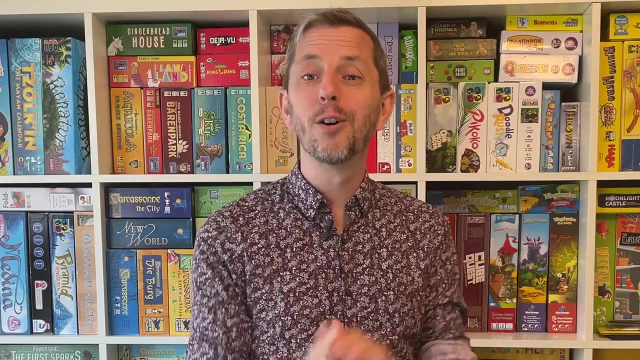 every aspect of my favourite video game. These days I stress out over sales figures, royalty checks and positive reviews and I wish I didn't Always remember the reason you got into game design and try not to lose the sense of childlike wonder Creating your first board game. 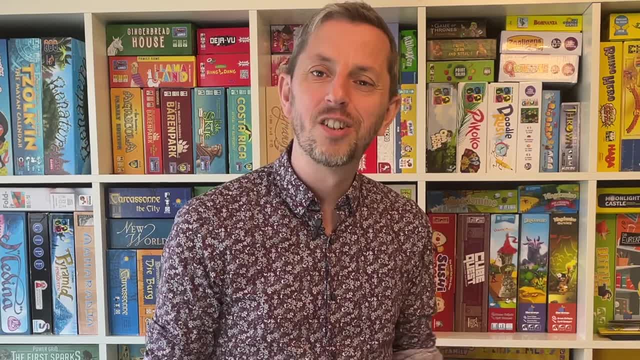 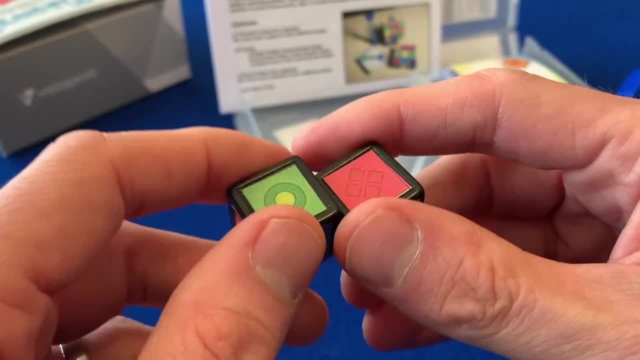 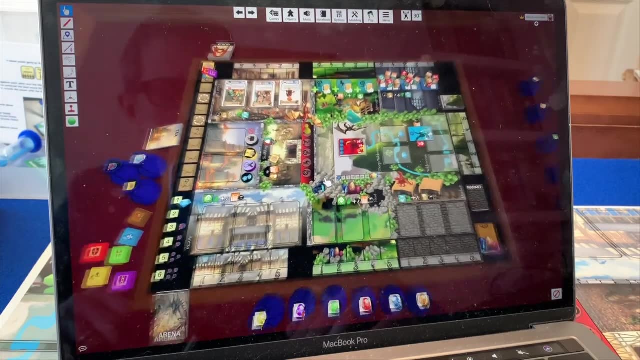 can seem like a daunting task, but with determination and a playful spirit, you can turn that squatter in your frontal cortex into a tangible, playable game. Whether you start small with a simple concept or dive headfirst into a complex, immersive world, the key is to keep in. 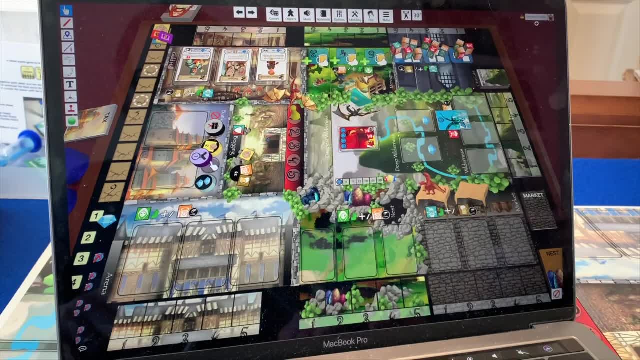 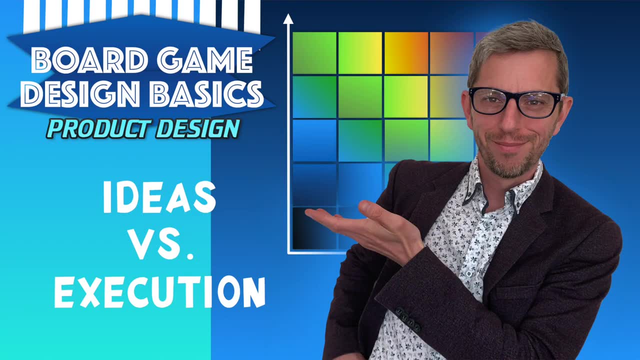 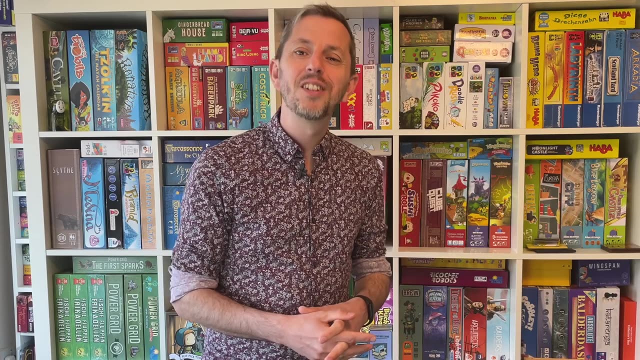 This has been a refreshing video to make. Most of the videos on my channel are focused on designing for commercial success, and that's a wholly different skill to what I've covered here. If you're interested in professionally publishing your games, I strongly encourage you to use a 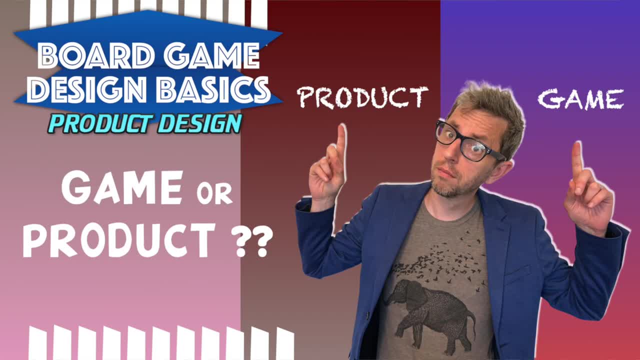 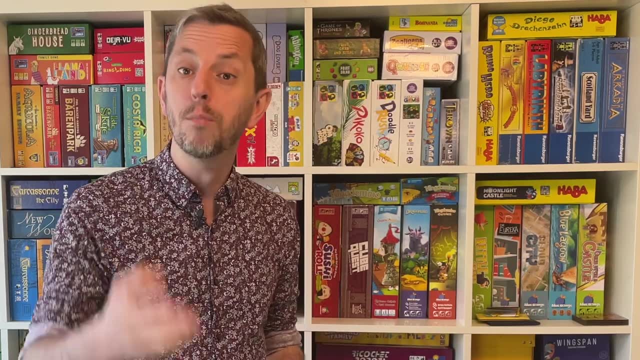 design-thinking approach: identifying a market, understanding it, recognising the player's needs, ideating solutions and then prototyping and testing rigorously. To learn more about this approach, follow the link. 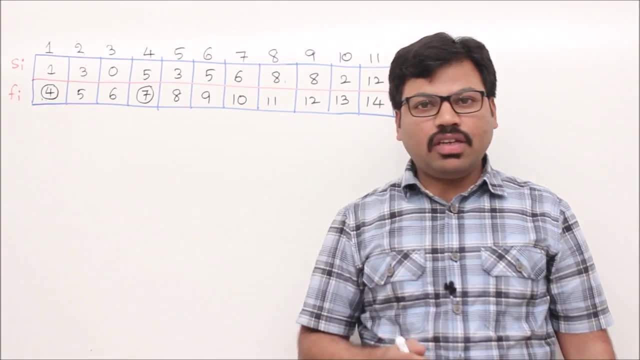 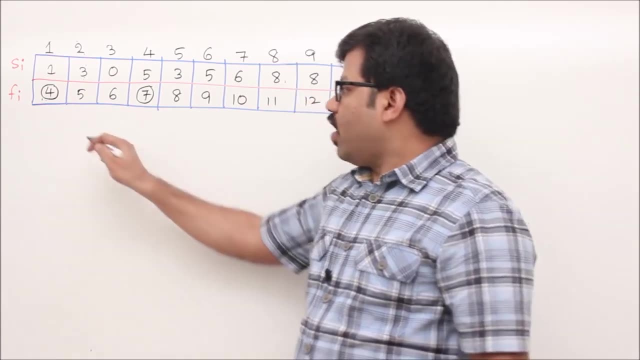 now we'll see greedy solution for this activity selection problem. so far, we have seen dynamic programming solution and it was very difficult, correct? but we can solve this problem easily using greedy choice. so what is the greedy choice here? i will tell you. so, in this problem, there is actually 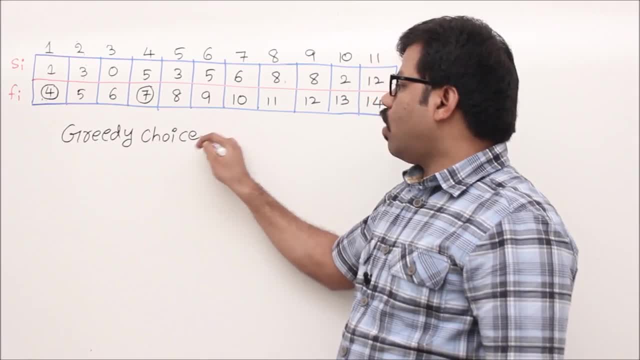 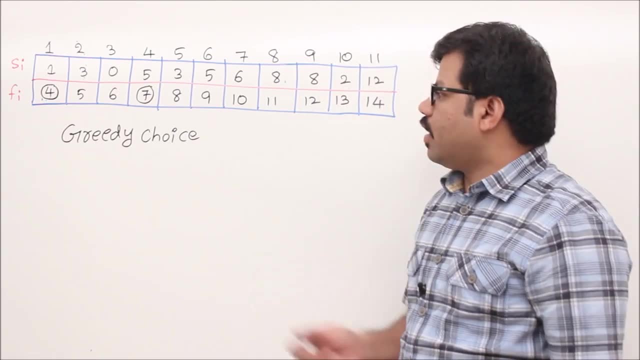 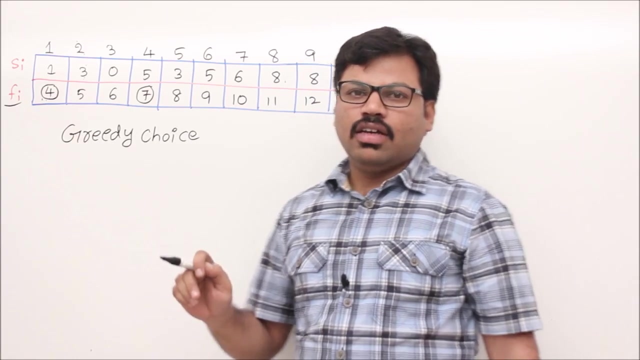 there is a greedy choice. that's the reason we can solve this problem easily with respect to, you know, problems, complexity at the same time, time complexity also. we will see that first. what is greedy choice here is first sort the data using finishing times. once it is done, then always pick.